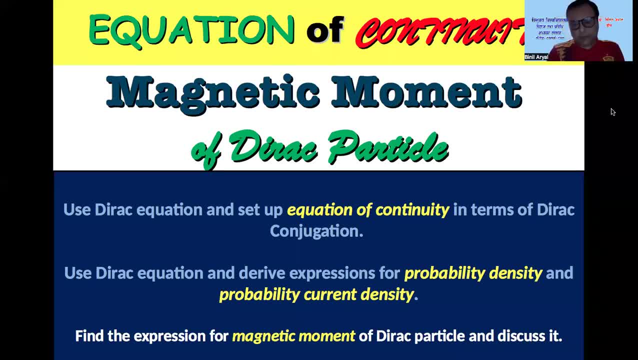 very high When it becomes relativistic. what will be the effect of turning Broadly? you can understand that there will definitely be a turning effect, which we will now do the derivation, But the magnitude of the turning effect is extremely small. 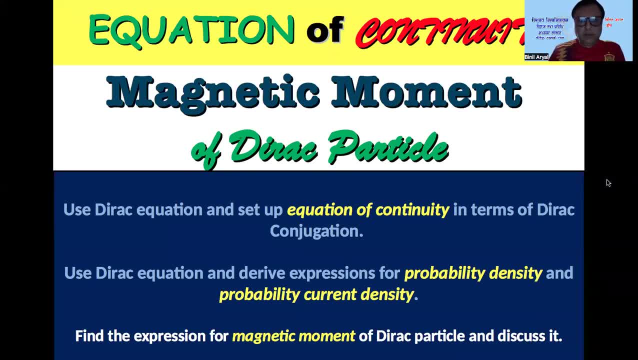 However, the particles of the turning effect are very small, The energy of the turning particle is very, very high And the interaction time, the interacting time, is extremely tiny. It interacts at very short intervals. At that time, no matter how small the magnitude of the turning effect is, it affects not only 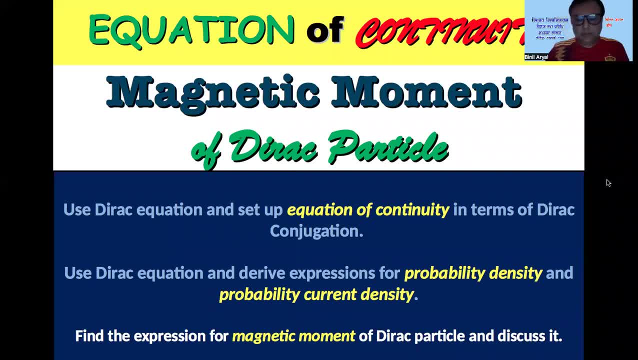 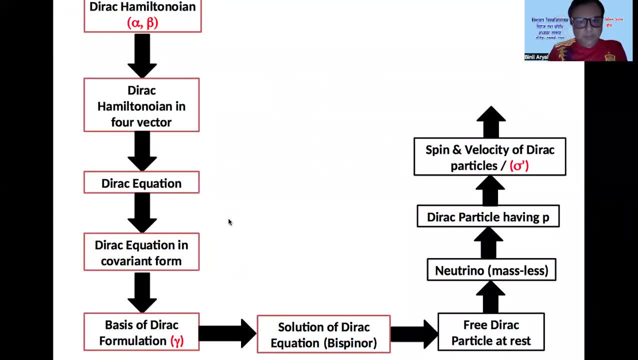 the detector design, but also the physical properties. What properties it affects we will learn in the next class, helicity. So today I will begin with these very fundamental things We have completed up to the point, completed up to this. We started from Dirac Hamiltonian. We discussed alpha and beta and 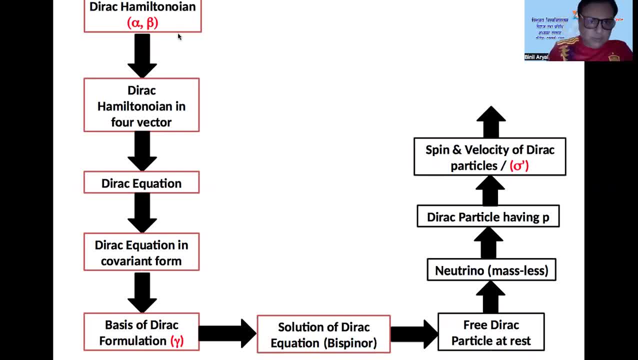 wrote the relationship in various ways between these two 4 by 4 matrices introduced by Dirac in his Hamiltonian And we also discussed- we also write Dirac equation in four vector form And we also discussed about the implications of Dirac equation. It's also solution And 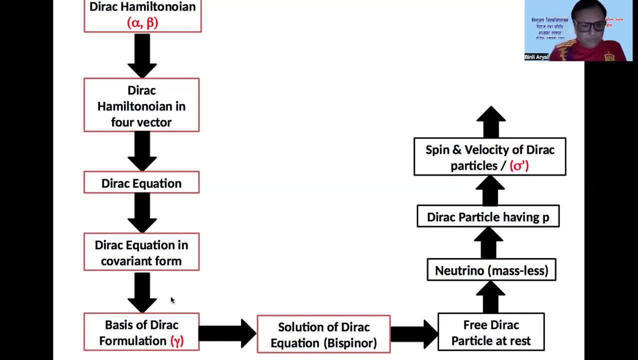 we have written Dirac equation in co-variant form as well. So also to do this we introduce gamma matrices. So these are the basis for Dirac formulation. So alpha beta were introduced and gamma matrices were introduced. Then we came to the solutions of Dirac equation in 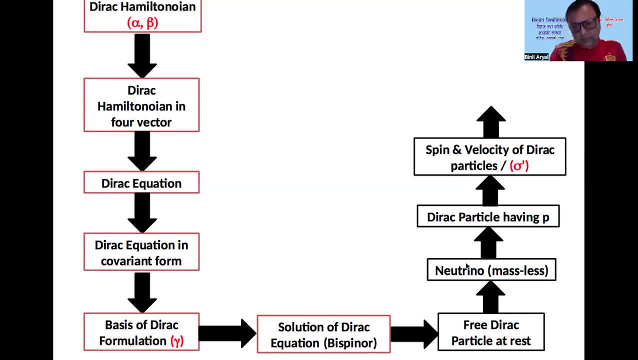 some cases Free Dirac particle at rest. neutrino Dirac particle having momentum B. Many people have not done this Until now it has been 20 years. So in the last class we discussed about spin and velocity of Dirac particle And here 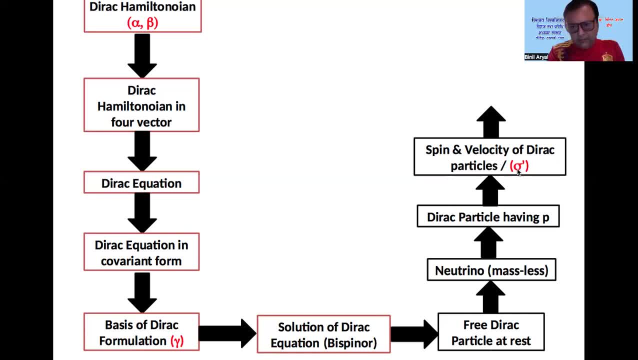 we introduced Dirac spin matrices. We introduced sigma prime. here We started with alpha and beta, Then gamma matrices became very important for us. Then in the last class we discussed spin. In the discussion of spin Dirac spin matrices were introduced. Then gamma matrices became. 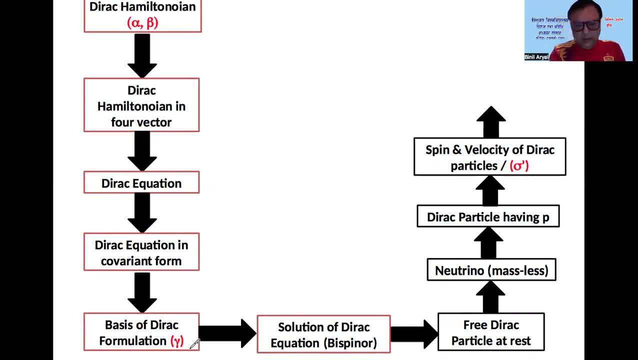 very important for us. Then in the last class, in the discussion of spin, Dirac spin matrices were introduced. Then gamma matrices became very important for us. Then the formula was introduced. Until today this is one special form. So here in this we write Dirac spin. 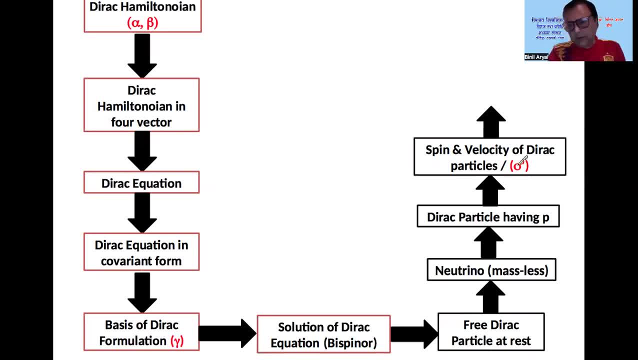 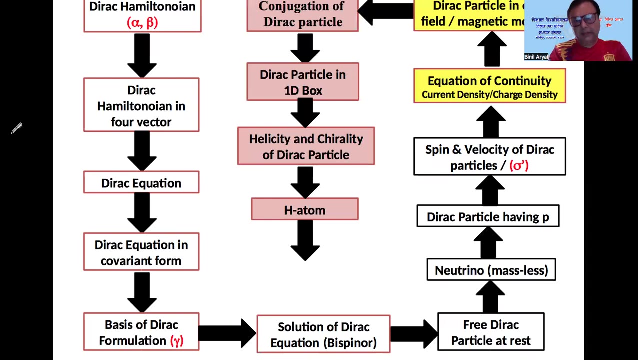 matrices, and we used this to find something that Dirac had assumed to define the spin of the relativistic particle, or at the intrinsic angular momentum of the relativistic particle. Now, that is enough for us. Today we are going to discuss the equation of continuity and the expression of current density discharge from the direct equation. 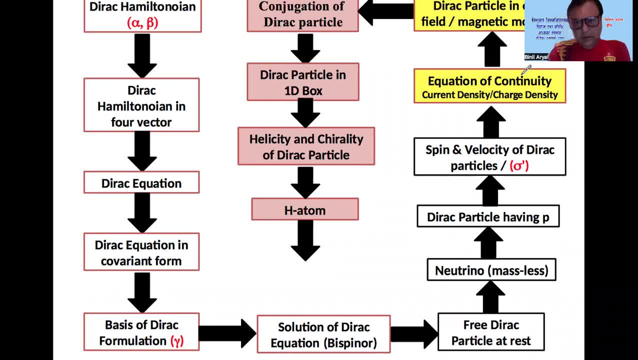 We will discuss the magnetic moment today. We will put the direct particle in the electromagnetic field and then we will check the accountability of the turning effect of the direct particle. And in the same way we will introduce some other matrices. We started from the alphabet, came to the gamma matrices and also did the direct spin matrices. 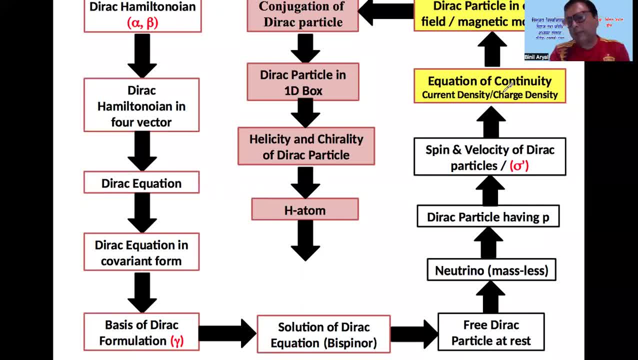 In other words, we have defined something else in direct conjugation. We have defined the conjugation here. We will use the conjugation here at the top and also at another point. At the same time, we will define the form of another matrix here. 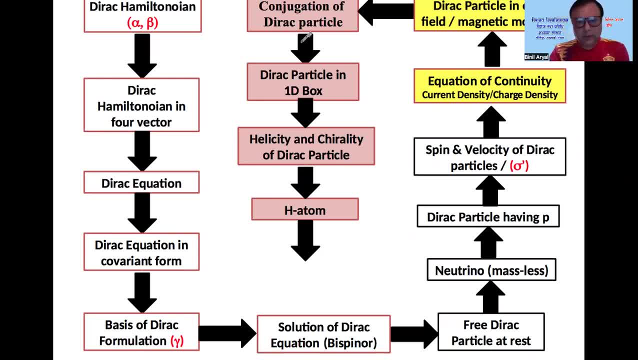 So today we discussed these two blocks And in the next class I will discuss conjugation of direct particle and direct particle in one dimensional box in order to compare with the classical result. So this is extremely important in terms of experimental verifications. 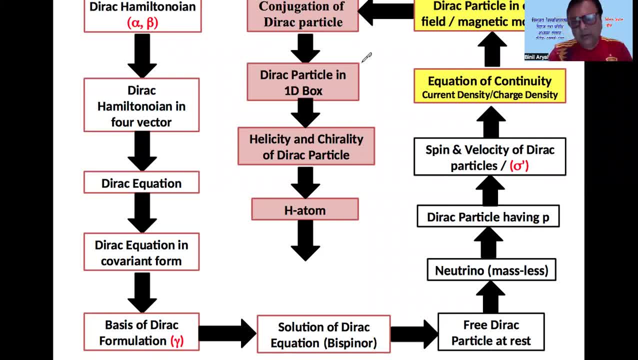 Your part is very important. We will establish it in direct formulation. Similarly, this part is also very important. We will establish it here as well. We had experimentally measured the anomalous magnetic moment. We had not redeveloped the theory of where it came from. 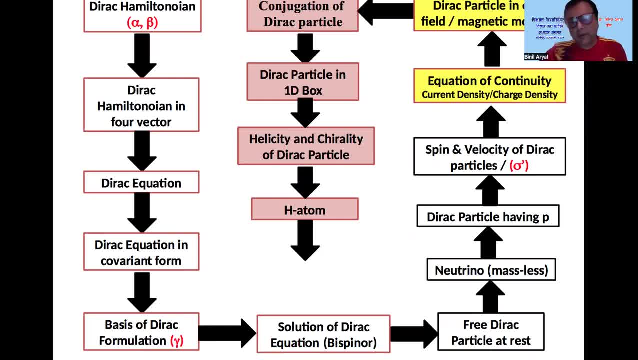 We will develop the theory directly. We had measured the turning effect of the reduced particle as well Previously in accelerators, cyclotroners and small linear accelerators, So we will try to complete these two sections in one class And I will take it for one class. 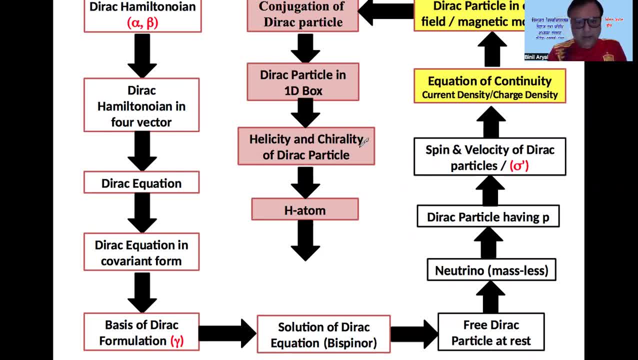 This is very important: Helicity and chirality property of direct particle, And this goes continuously to the hydrogen atom problem. This is itself. If you do it in one class, you can discuss it in two hours. These are connected. somehow We will come up with these steps from here, not from the helicity. 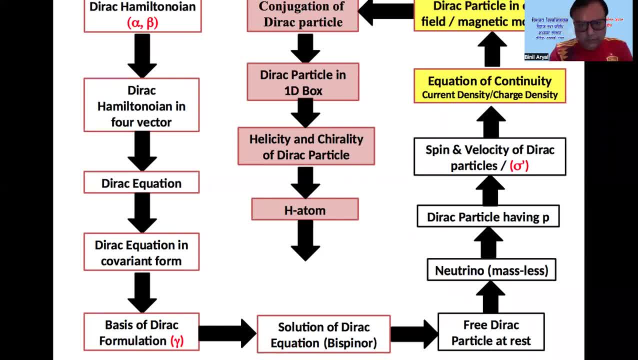 We will use the full potential of hydrogen atom. We will use the standard equation, differential equation. We will write it down. So these two are relatively isolated to each other. So this can be connected. These are not very weak. These cannot be asked as long questions. 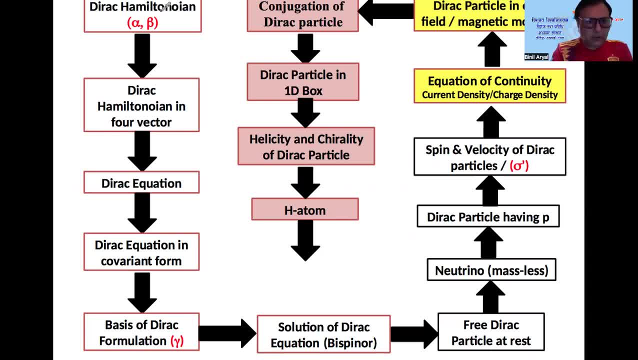 This portion is important for long questions. This portion of direct formulation is important for long questions. The spin and velocity are also important for long questions. The solution of direct equations, The solution for direct particle having momentum, P as well as mass, both. 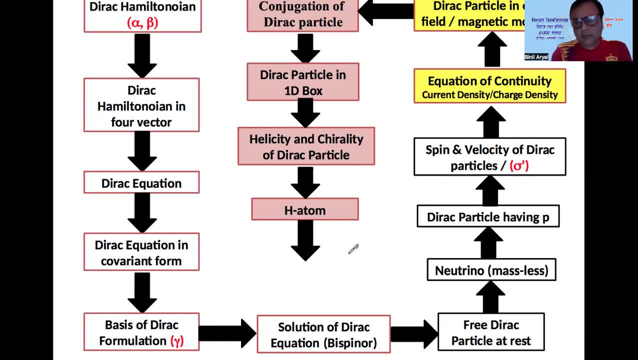 That is also a long question. Other things are small questions. After that, the direct field with the union. Dhani Raj has studied the direct field and the interacting field And Narayan sir has studied the field of Klein. I don't have time for this. 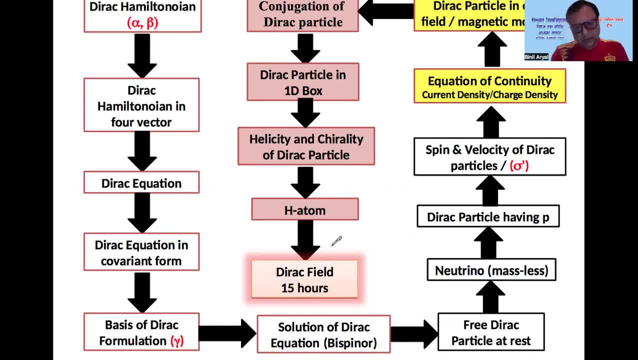 I would like to complete this in two classes, If possible. after the final term exam, you will have to study the final term. If the course is good, you will know the problems there. After that, after the final term, I will only have a general discussion about the field. 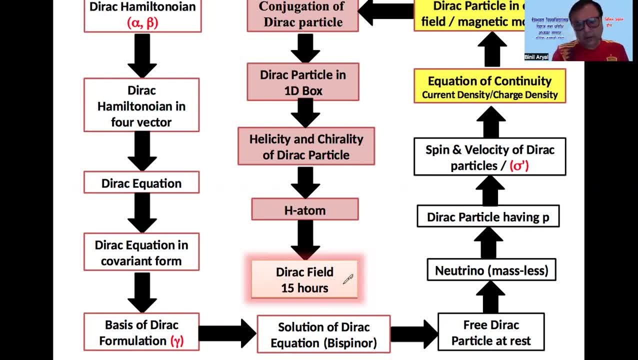 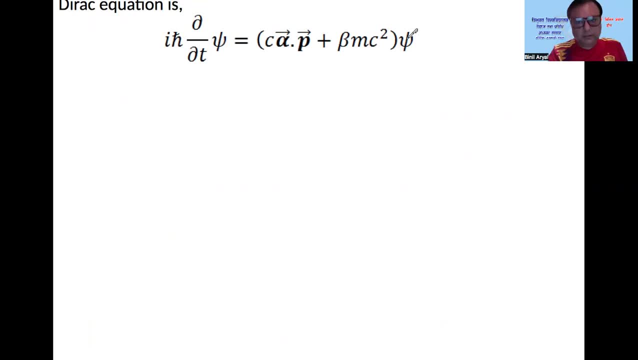 I have not read any other things. I will have to interact with them. Okay, So let's move to equation of continuity. Okay, This is direct equation. You know this. This is i h square d psi by dt h psi. 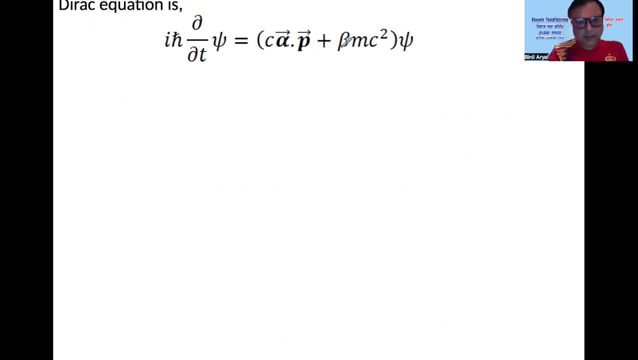 So h is this direct Hamiltonian in terms of alpha and beta. So I have started from this, Even if you want to know where to start from, if you want to go through classical analog or if you want to go through non-realistic analog. 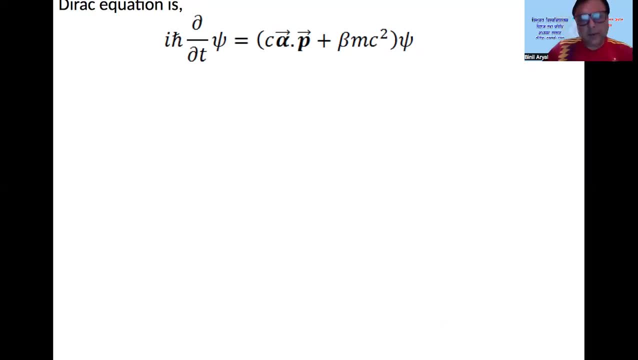 generally, this equation starts from direct Hamiltonian. But if you want to go through relativistic, analog, if you want to go through relativistic, it starts from the direct equation in the form of four vectors. And if you want to go through the field, 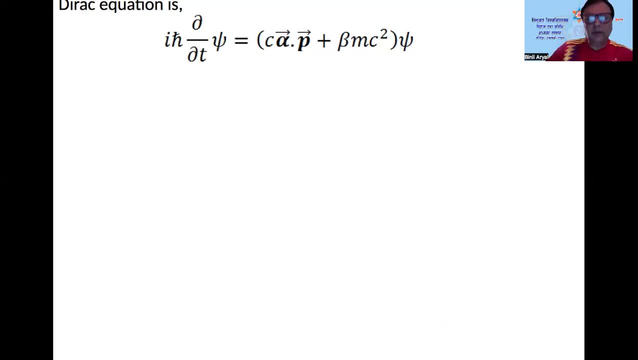 it depends. It can be this way: If you want to go through the properties of the field, it starts from the form of four vectors. Generally, the properties of the field are established in four vectors. This is how it starts. So here this is direct equation. 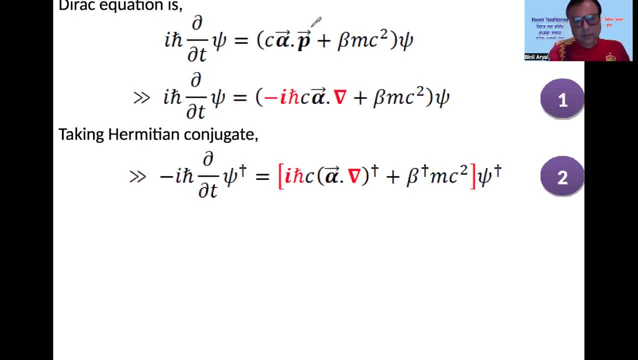 So you know this Momentum should be treated as an operator. So I replaced momentum p, considering it is an operator, by i h square del. So this is your direct equation, And now I am taking Hermitian conjugate of direct equation. 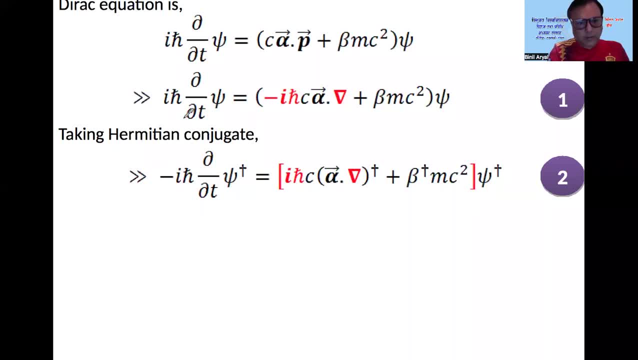 So I am taking complex conjugate Or, in a better way, I am taking Hermitian conjugate of direct equation. First I am taking psi and then I am taking dagger. So here you have i, So you have to take. 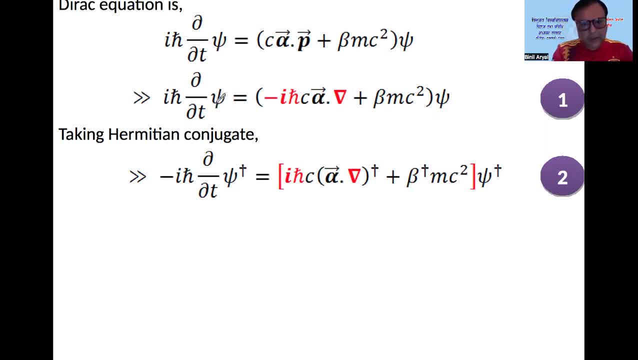 you have to make it conjugate minus And you have psi, So psi dagger, And also here you have i, So this minus becomes plus, And also you have, say, this operator, So you have to make it conjugation. 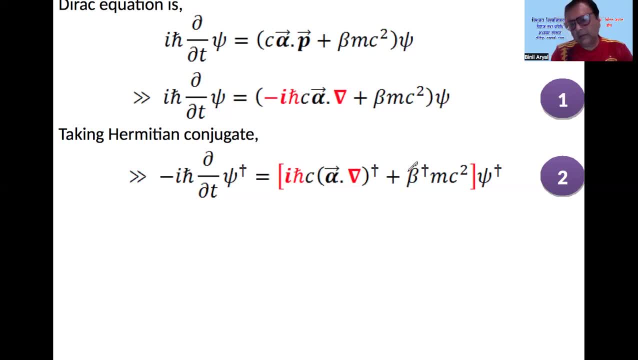 Make it conjugate, And also for this matrix And also obviously for. So this is the Hermitian conjugate of direct equation. Then what do we do to get equation of continuity? In this upper equation we multiply by psi, dagger. 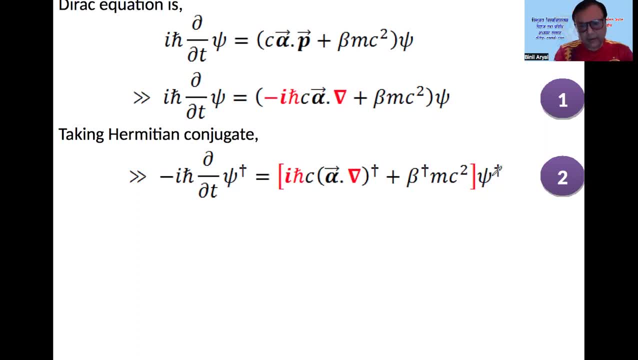 In the lower equation we multiply by psi, by wave function, Right From the same order, From left from right, Then we subtract from this, Or we subtract from this, We take conjugation, We multiply. Wherever we do this, 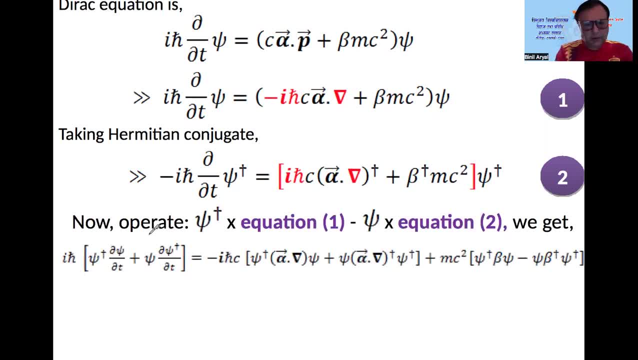 we do the same. So okay, Now we operate, operate equation one by the psi dagger and equation two by psi, and subtracting in this fashion. So you get this Okay. So here you know. beta is the temporal part. 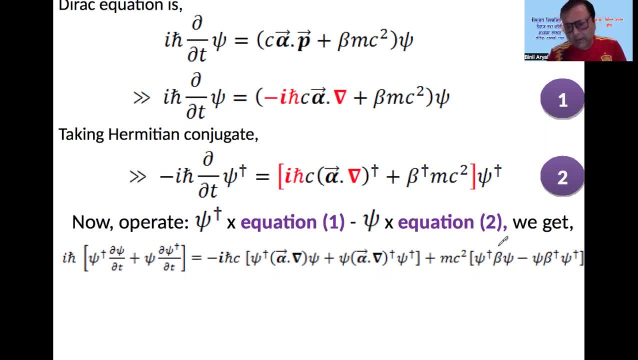 of the introduced terms introduced by Dirac. Alpha is spatial part, So beta gives a number, It is actually a number. So this term reduces to zero Your part. This term reduces to zero because you know, beta equals to beta dagger. 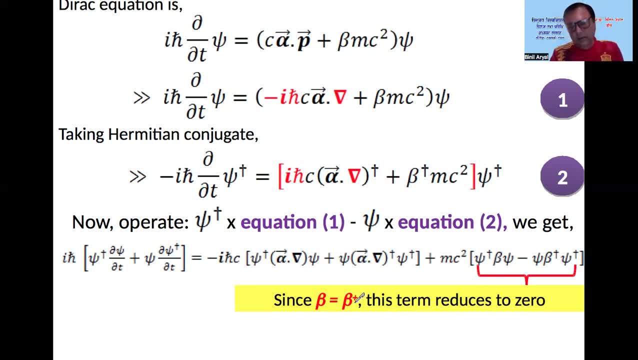 equals to beta. inverse equals to beta is gamma four. Gamma four is Inverse of gamma four is gamma four. Adjoint of gamma four is gamma four, And its covariant and contravariant are also the same, So this term reduces to zero. 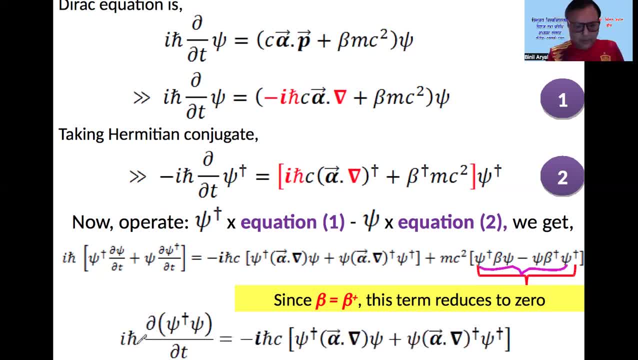 You have only plus two term. Now here you know, i has got d psi by This probability is the value by dt. Well, a del dot. something has to be kept in the form of the equation of continuity. Here there is one problem. 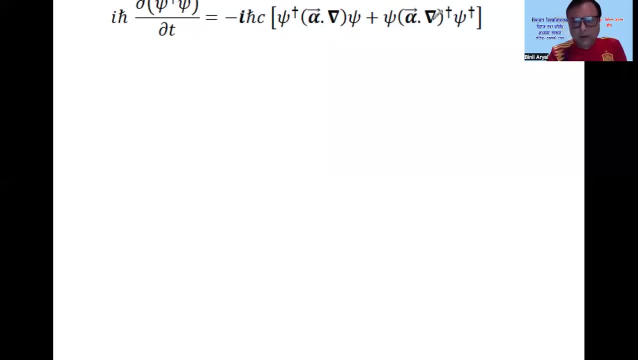 If we look carefully here, this alpha dot del has a dagger in the whole operator. Therefore this dagger has a dagger along with alpha Here. there is no dagger Here. psi dagger is psi Here, psi is psi dagger. 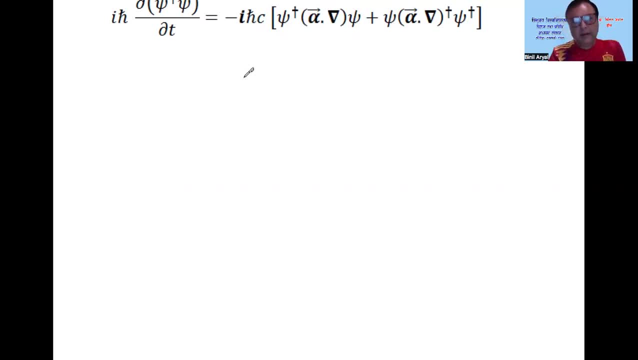 This is fine. If we take out the del, we have to keep del dot something. This is the current density. Now we have to make this assumption Here. I have just i has got, i has got cancelled. I have just simplified it. 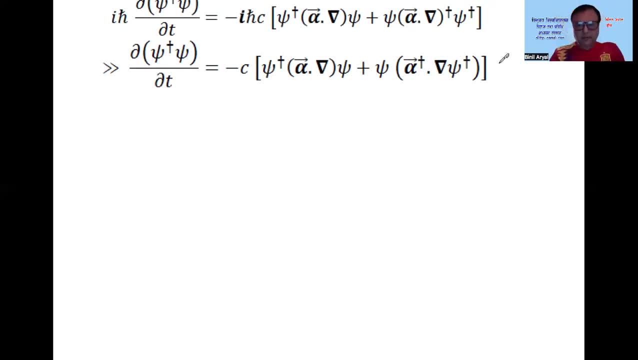 I have just cancelled, i has got. The rest is the same. Now, here, I have alpha as alpha dagger. You have alpha here, You have alpha dagger here. Okay, Now, if we make this assumption, then only the equation of continuity. 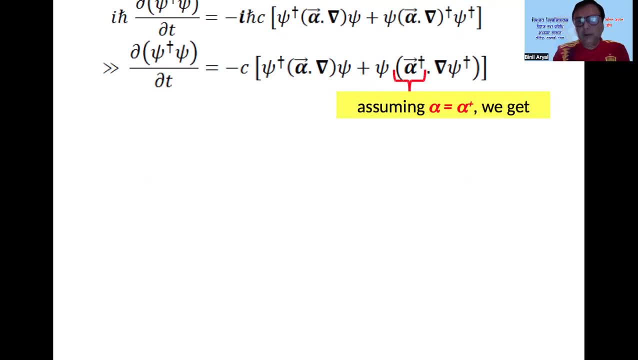 will be possible. Okay, So let's assume. So we will discuss. what are the implications? Let's assume alpha equals to alpha dagger, Beta equals to beta dagger. that you can prove using matrices. But here, if you look at the matrices, 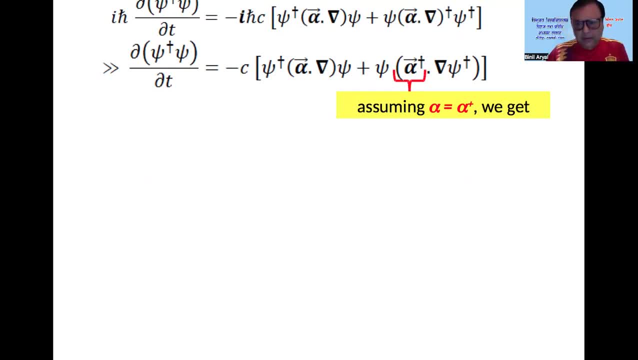 of the alpha, alpha x, alpha n, alpha z, then the alpha is not always alpha dagger. Only under some conditions alpha can be alpha dagger. So here we have assumed alpha equals to alpha dagger. So we deploy the conditions. 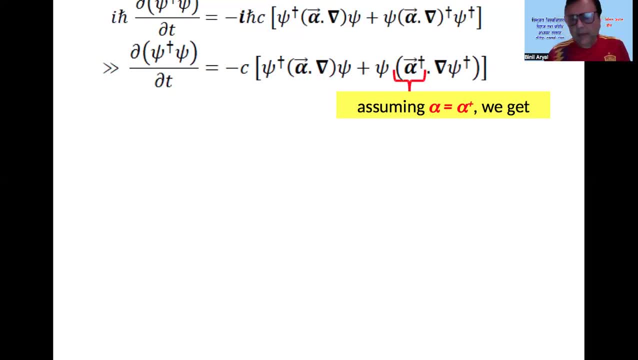 that compel these matrices, matrices of alpha, alpha x, alpha n, alpha y- to be alpha dagger. Okay, We deploy that condition. Let's assume alpha equals to alpha dagger Mathematically. If we do this, then your equation takes this form: 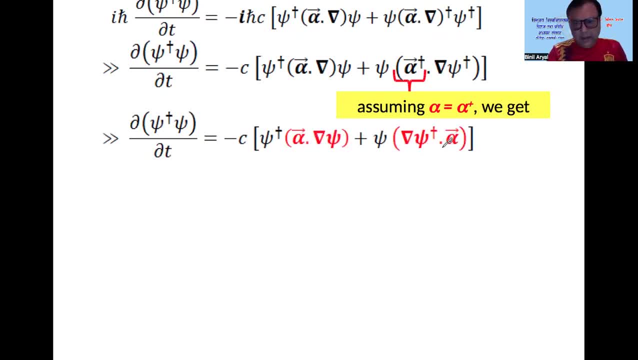 alpha dot del xi, del xi dot alpha. Here we call the dagger as alpha. only This equation can be written in the form of continuity. So here this is nothing. This is del dot. If you differentiate it, it will have two terms. 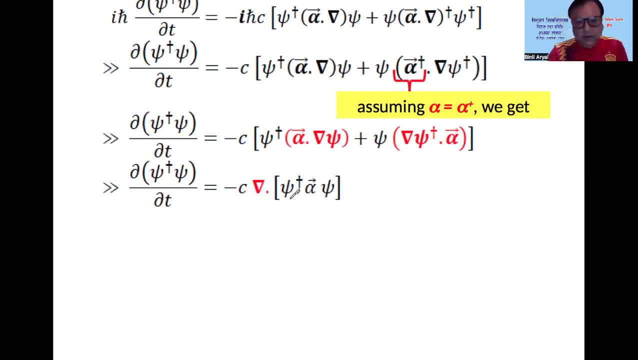 Exactly this one. So del dot xi, dagger, alpha xi, So you will have this. So if you take it here in this side, left-hand side, you have this form. So this form is more or less similar to equation of continuity. 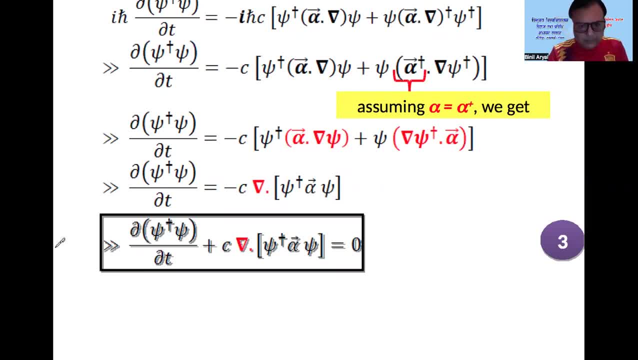 that we have in discussing non relativistic quantum mechanics. So this is priority density and this is somehow current density. You see, including xi, Including xi. So here these two terms are similar to current and priority density. So comparing this equation, 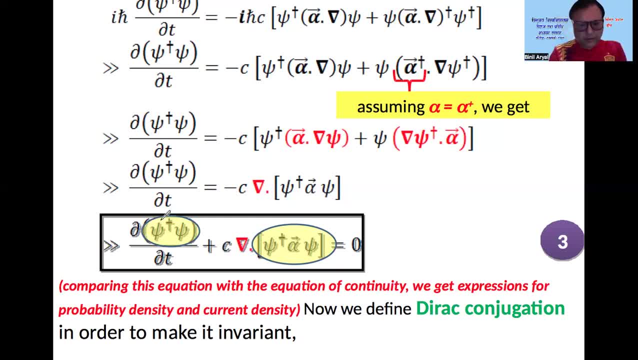 with the equation of continuity, we get expressions for priority density- This is priority density, and current density- This is current density. But what we are doing here is we define a new term that is called direct conjugation in order to make it invariant. 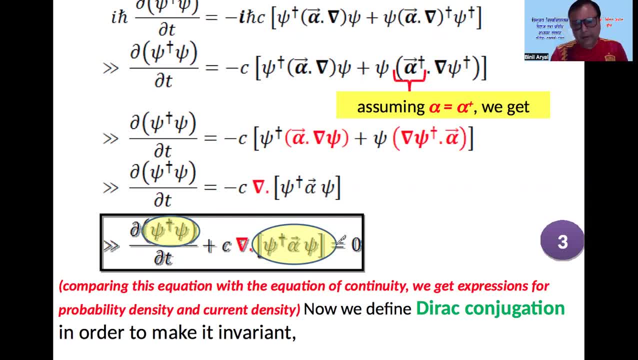 Relativistically, we have to write it in four vectors, Right, But in this way we can understand that we have written this by assuming this. Okay, So let's introduce conjugation. conjugation for the solution of direct equation. 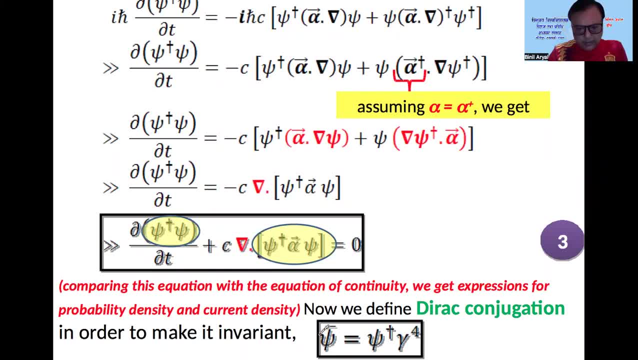 The solution of direct equation is the general solution for the direct particle. This is the function. We put this bar above and call it conjugation, And we define conjugation like this: Xi, dagger, gamma, 4.. Gamma 4 is beta. 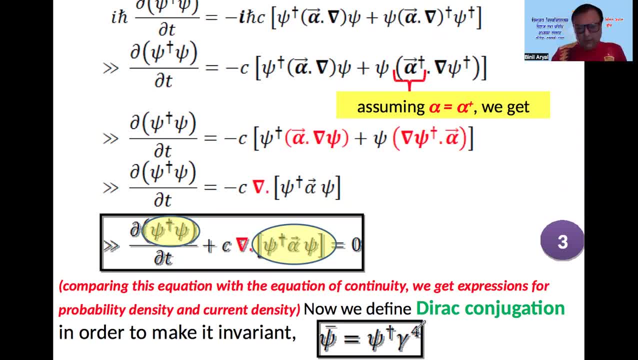 You know this. And this is equal to inverse of gamma 4 or dagger of complex conjugate of gamma 4.. So you have multiplied with conjugation in order to define this conjugation function. Okay, I will introduce conjugation here. 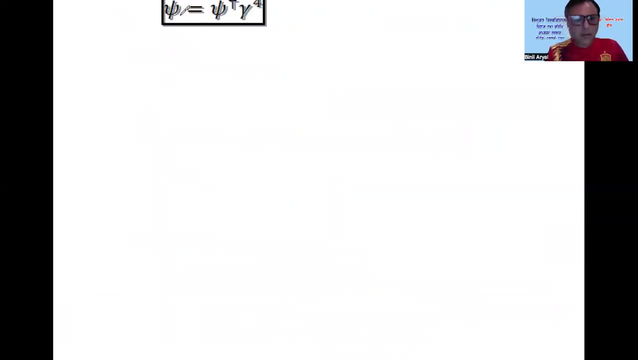 Look at this bar above. Okay, So you know what is gamma 4.. Gamma 4 is this: is the function of direct equation. Okay, So you know what is gamma 4.. Gamma 4 is this is this: is say the 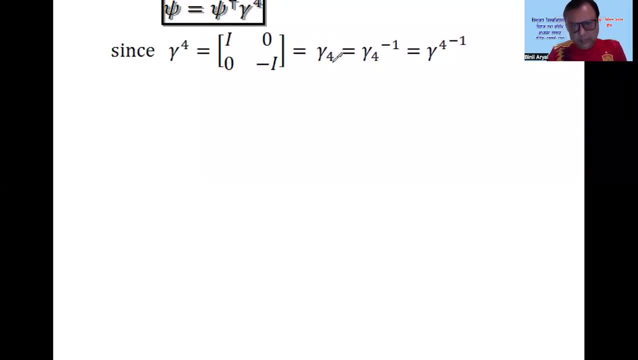 contravariant Gamma 4 is gamma 4 or inverse of this gamma 4, or inverse of upper indices with upper indices of gamma 4.. So gamma 4 is because this is this matrix, You can do this and you you know. 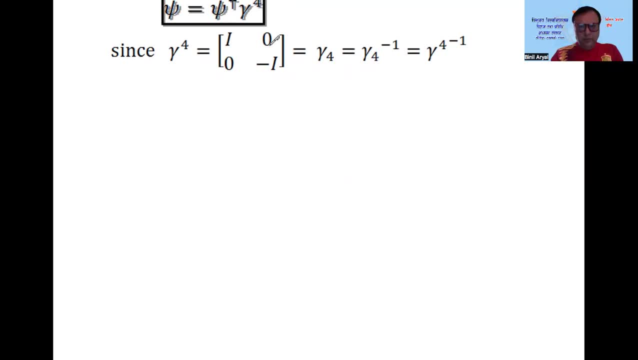 this is 4 by 4 matrix, So this block contains 2 by 2 and also this block contains 2 by 2.. Okay, You know the relationship of gamma 4.. This is so you can take it out. 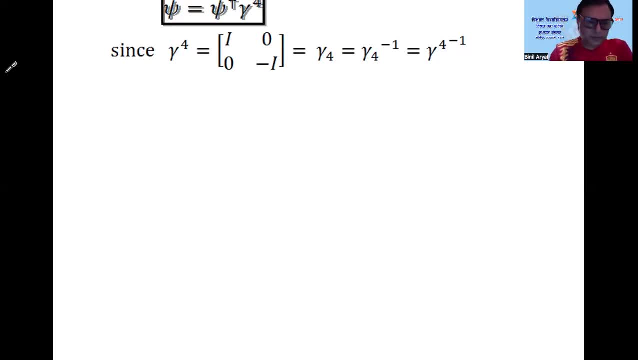 You can take gamma 4 and put it here, because its inverse is the same. Okay, So if you do the same gamma 4, I will keep it here. So side dagger equals to conjugation gamma 4.. Okay Now 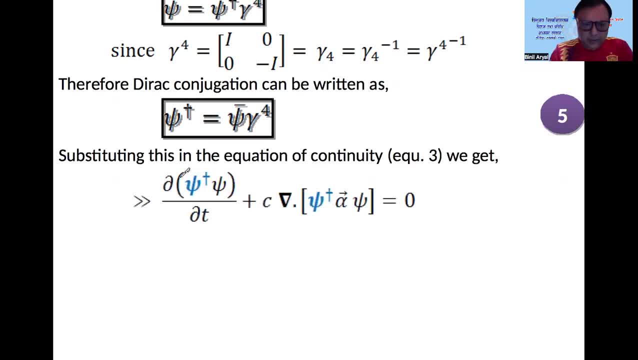 our next equation is the equation of continuity. We wrote this as priority density and this as current density. We have conjugation in both places. Right, We have side dagger in both places. We have defined side dagger in terms of conjugation. Now, 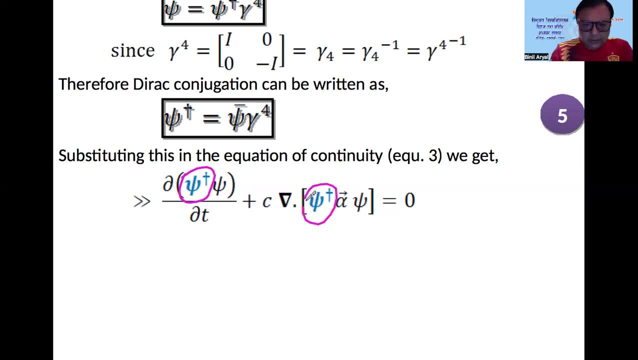 we substitute this side dagger here: Okay, Okay, So this is conjugation gamma 4.. We write conjugation gamma 4 here. We write conjugation gamma 4 here: Gamma 4, gamma 4.. There are two of them. 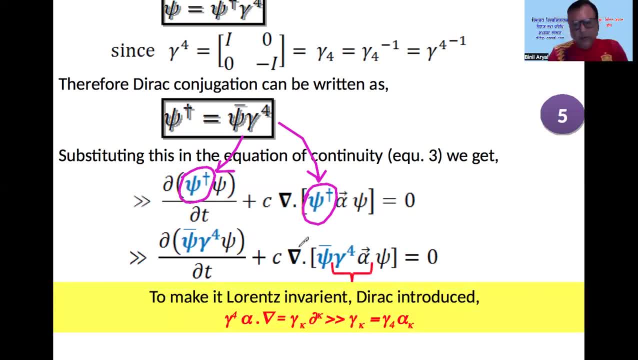 Now gamma 4 and the production of alpha contains three components. There are three of them. It has three components: x, y and z. So it has the temporal component. The fourth component is here. The product of these two is 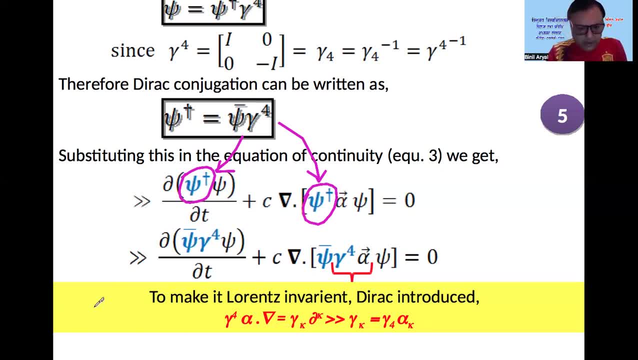 gamma matrices. Just to recall, I have written this line To make it Lorentz invariant direct slide. I had introduced this form. And gamma k is gamma 4, alpha k When alpha is applied to gamma, gamma 4 is. 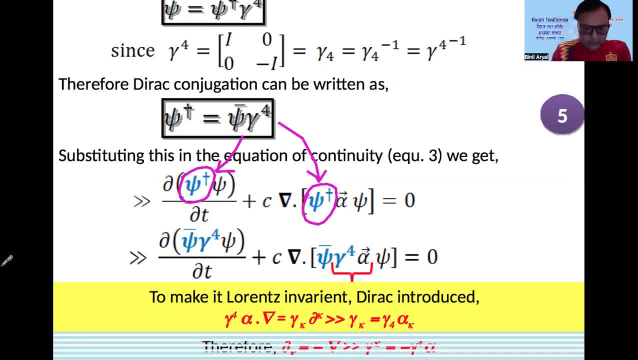 multiplied or operated in the matrix. So what we know about other things is that gamma k is basically similar to minus del. in mathematics We generally write del in four vectors. Similarly, gamma k has also three components And gamma k is again. 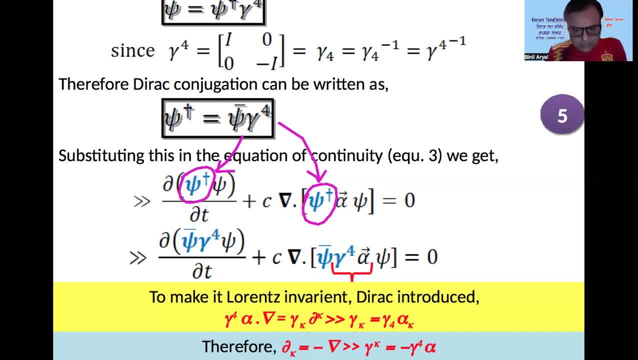 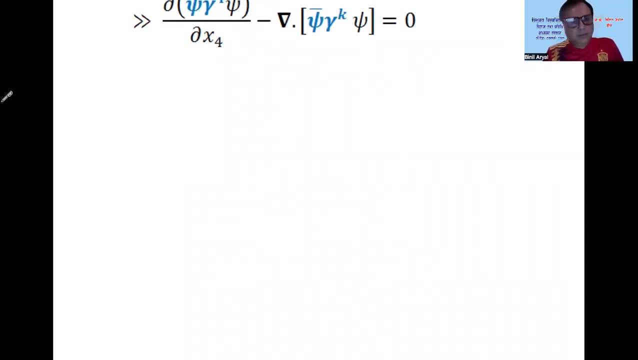 a multiplication of the two vectors. So this is the same form of conjugation that we discussed in the last video. We have not inserted that in the last video. Now I will show you how to write a two-dimensional matrix. So 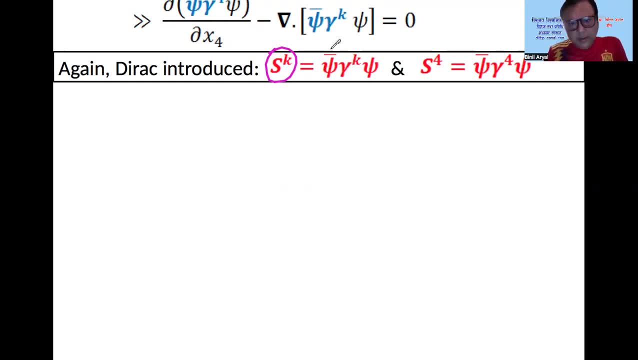 let's say this is the first square in the matrix, So we have to write the two squares of question of continuity in the middle of conjugation and wave function. we will introduce the spatial part. only Temporal is written separately like this: 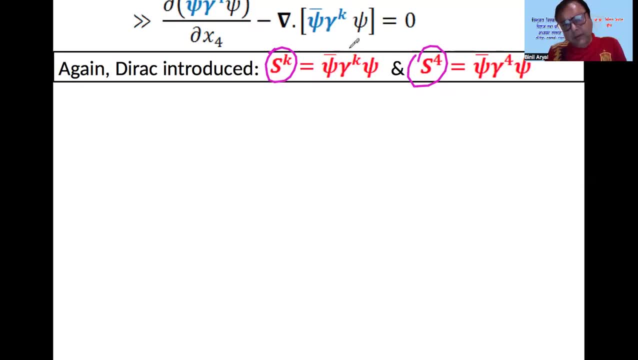 This is S4.. S4 is gamma 4.. It is not for three, So you can also write S new equals to conjugation, gamma new psi. And we will introduce it like this: Look here, Here is temporal, Here is spatial. 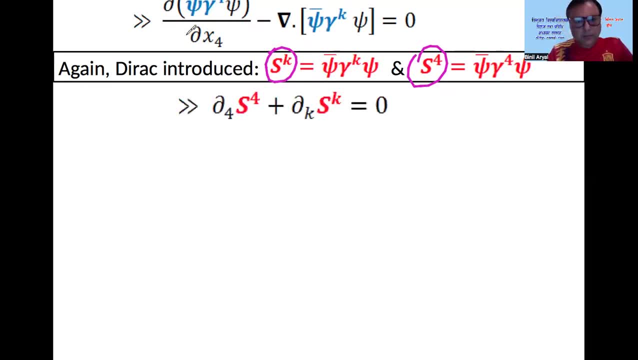 So, introducing this, what do you have? You have simply d by dx4 is d4.. And you have this: This is for S4.. d4, S4 plus dk Sk. So it has three components. It has the last component, or the temporal component. 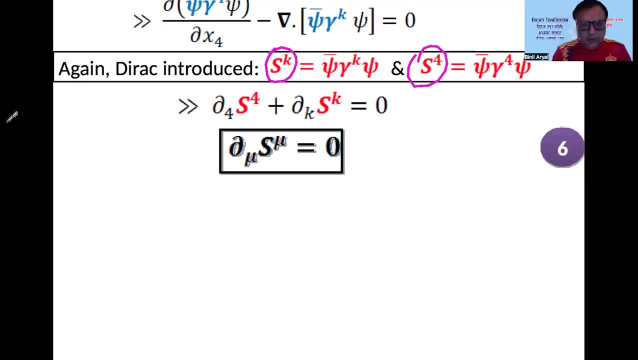 This is actually equation of continuity for direct equation for direct particle Del new, S, new equals to zero. So what is this? You know What is conjugation. You know This conjugation we already defined. So this is equation of continuity. 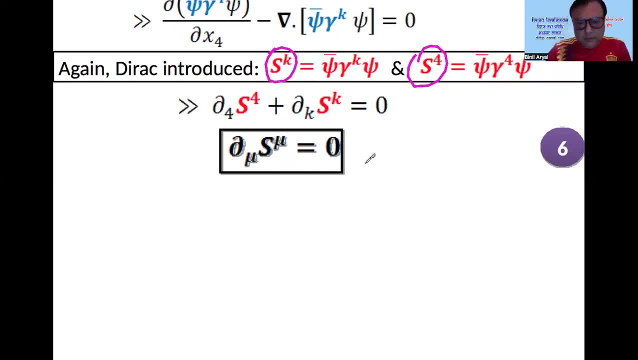 I mean, I suppose, discuss and derive or discuss equation of continuity for direct particle, Yes or no? I mean look at this. So this equation is called equation of continuity for direct particle in four-vector form, which is relativistically invariant form. 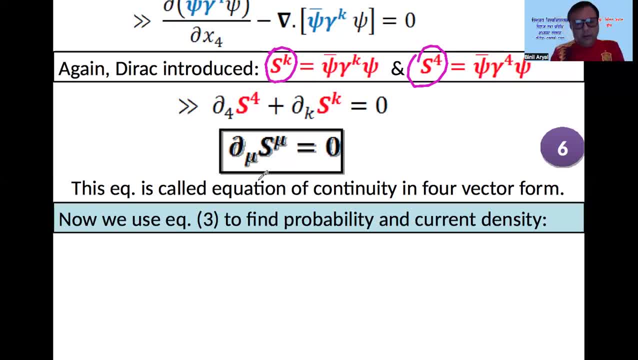 Okay, Now we have to find the expression of current density and probability density. When we solve the problem, when we find the probabilities and values of the current behind the particle interaction, which equation will we use If it had come before this? 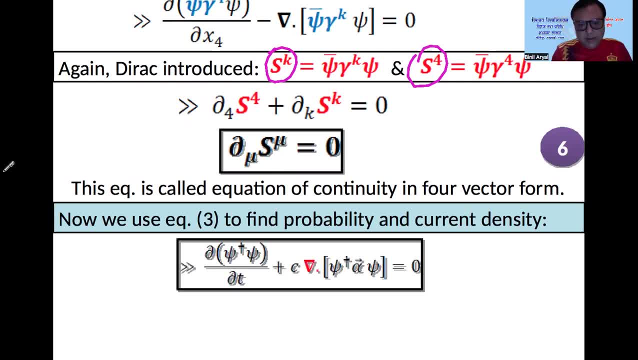 then this form or the form before this. we will see the previous form. In the previous form we introduced the conjugation. Okay, Let's now use equation three to find the probability and current density. So if you compare this with equation of continuity, 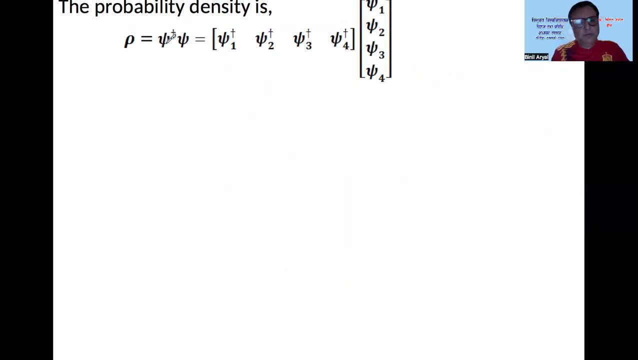 you get this. probability density simply is psi dagger psi, So psi dagger is. you know this is psi one, psi two, psi three and psi four. Direct equation to energy straight: plus or minus spin up or spin down. there is a possibility. 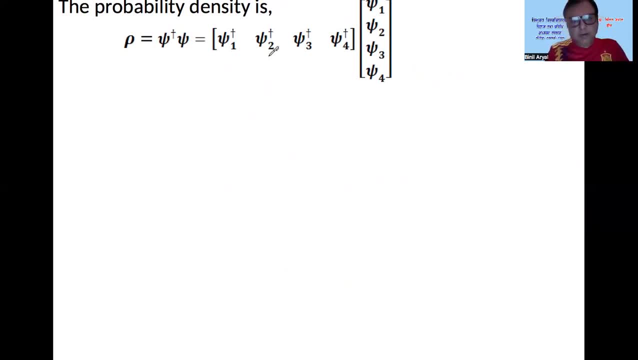 You know this. the nature of the general solution should have four components. So this is for the conjugation and this is for the this where general solution of direct equation, you have to write it in ket, in front the bra part. 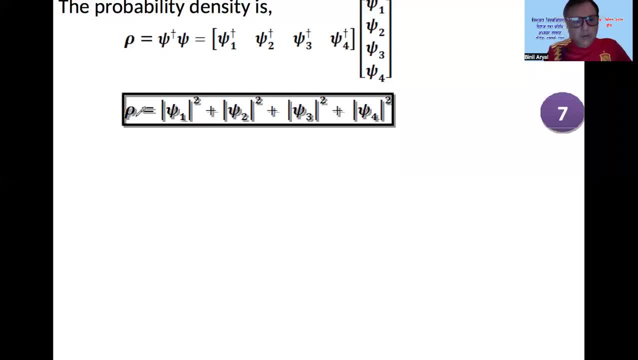 So if you multiply these two, you get probability density as psi one squared plus psi two squared, psi three squared and psi four squared. So probability should be positive, should be finite. So you can interpret this and this is not. this is very straight. 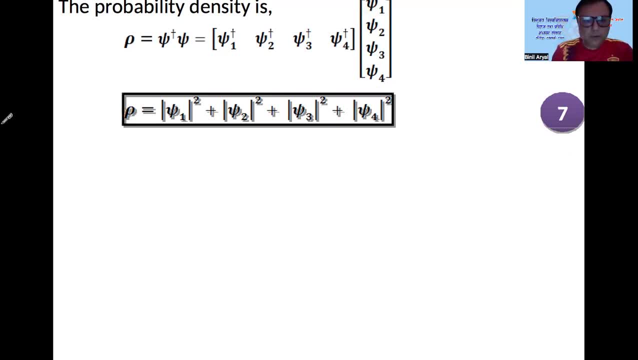 This is. there is no such problem, as you observed in the case of Klein-Gordon equation. So probability is finite and positive Similarly. so here it is written here. therefore, probability density of direct particle is always positive, like shown in the picture. 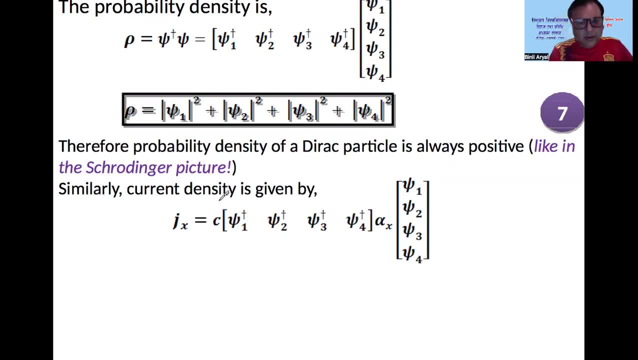 Okay. Similarly, if you look at the current density, current density in that equation, c, psi dagger, alpha psi, right. So psi psi dagger is in bra. so here you have ket and you also know alpha x matrix. This is for yux component. 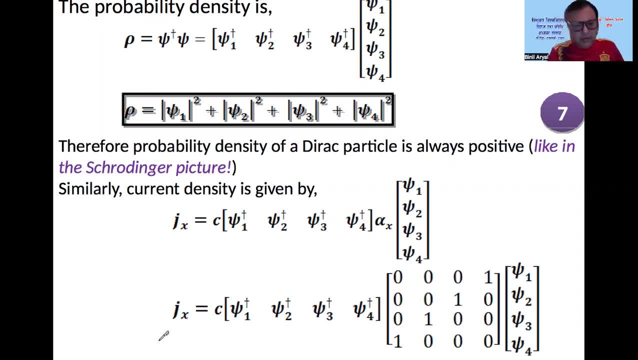 So if you calculate the current density for yux component, you have to put alpha yux, this is alpha yux, this is alpha yux matrix. And if you multiply these two and finally, if you multiply it with first, if you multiply three matrices, 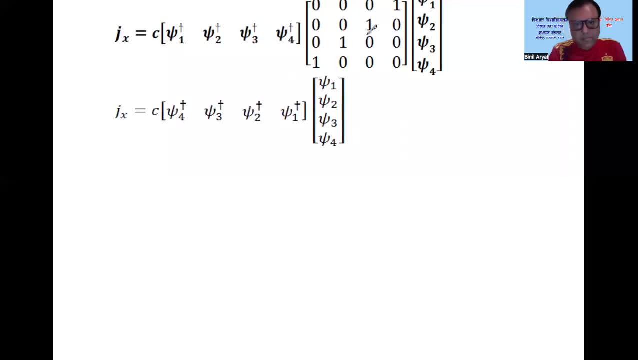 you get. you multiply this in: up: diagonal, cross, diagonal element, one side right, This will be psi one, psi two, psi three, psi four, this one also okay. Psi four dagger, psi four, psi three, psi four dagger. 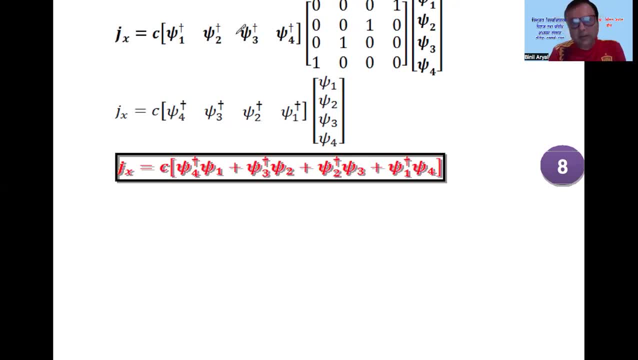 this whole thing. Okay, If you multiply these two? okay, I have done in this way. Your yux multiplied, right? Sorry, We have multiplied these two at first. If you do this, you have a cross diagonal here. So 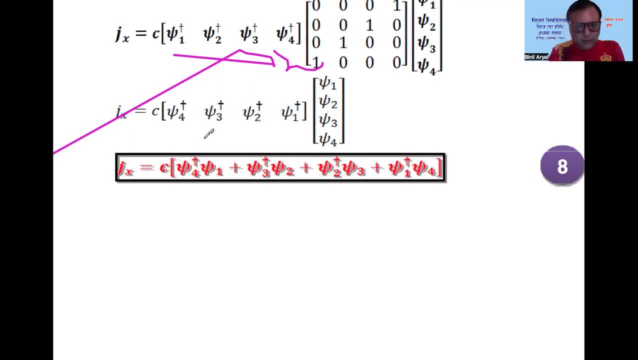 it's just reverse: three, two and one. Again, you can multiply these two. You have current density, x direction as this: psi 4, dagger, psi 1, 4, 1, 3, 2, 2, 3, and 1, 4.. This order with the 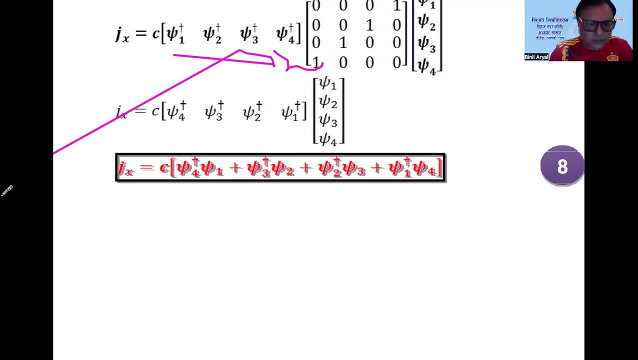 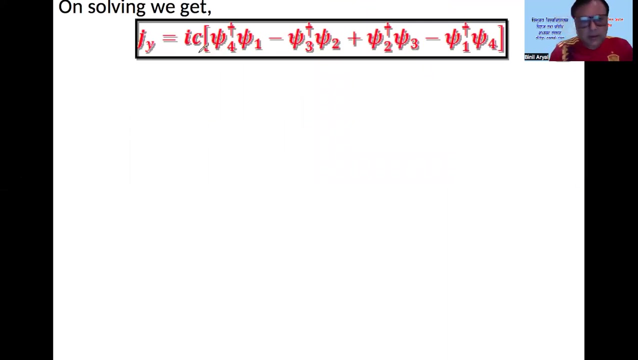 dagger. This is the expression for current density if the direct particle is moving along the x direction. Similarly, if it moves along y direction, you have to take alpha y and you know the matrix for alpha y. So this is the expression for j, y, So you have more. 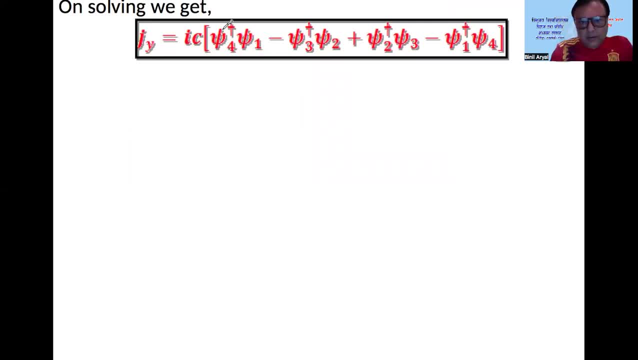 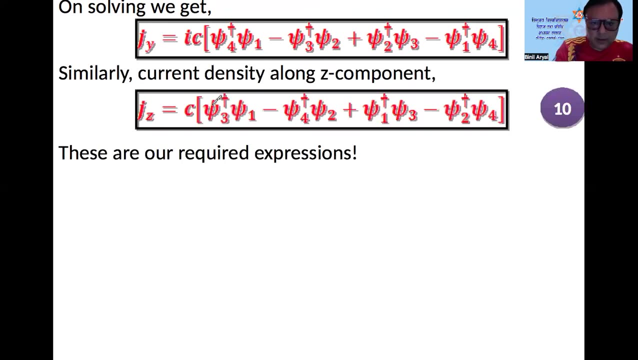 or less similar form, except the sign. So here you have additional i common, because it is obvious, This is the y component. Similarly, if you do this for z component, last component- you get a little bit different form: 3, 1, 4, 2, 1, 3, and 2, 4.. You see these three. 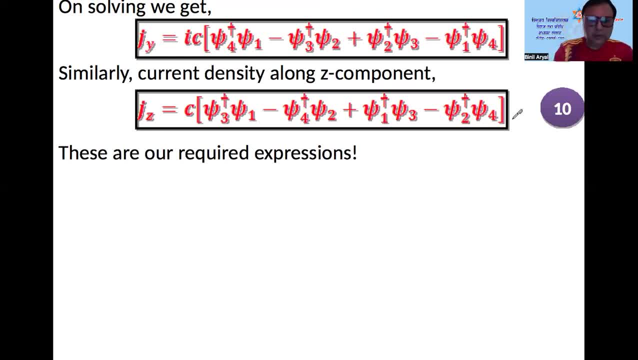 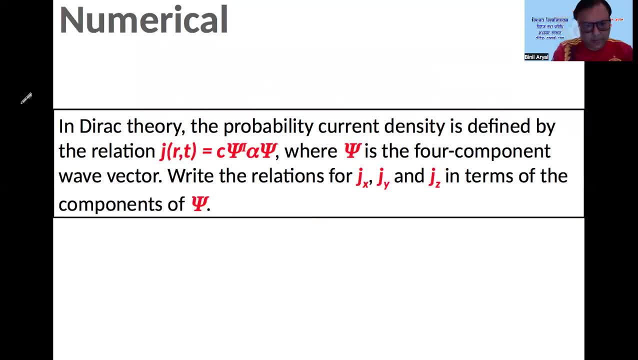 equations are very important to calculate the values of current density. 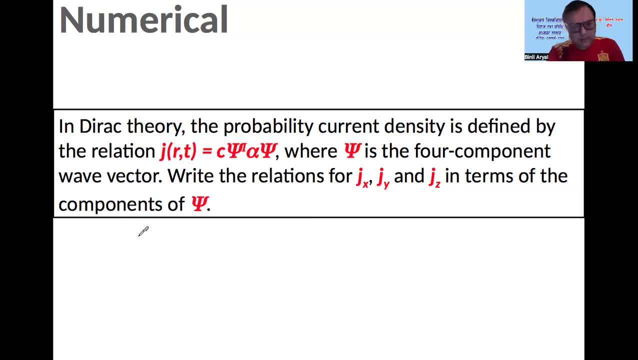 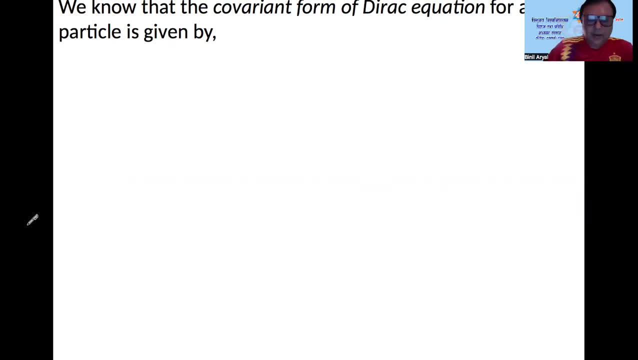 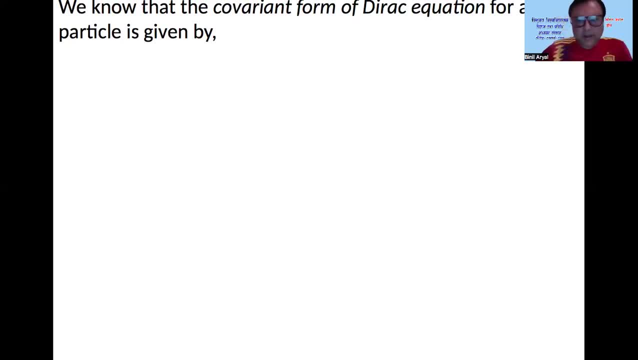 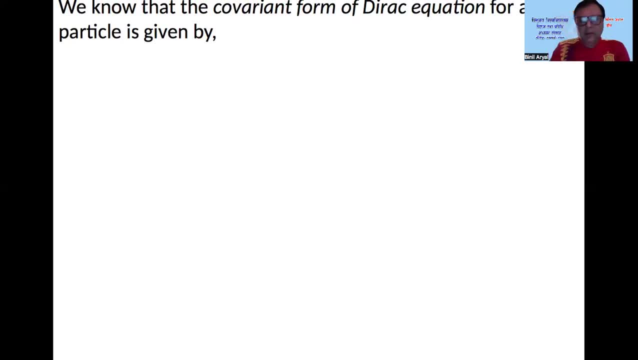 in the absence of electromagnetic field. if you apply electromagnetic field, the effect effective. 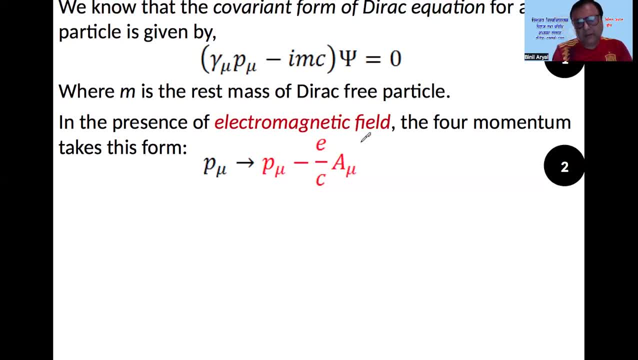 momentum will be reduced by this factor, reduced or becomes effective by this factor, because if this factor becomes negative, then this will be more than this, yeah, positive within the more than this one. so so generally this is effective. generally it is negative for fermions. okay, so you know what is a and you know the relations that you have used for vector potential, a and. 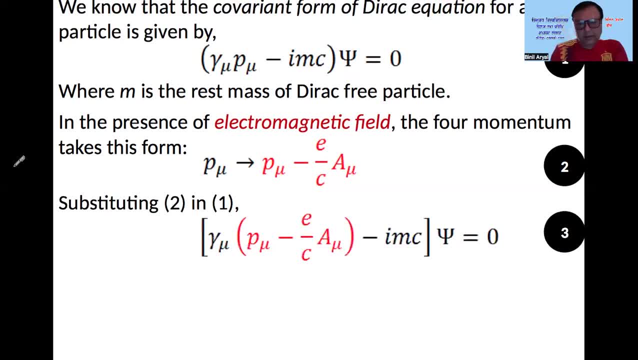 also the four vector form for a and phi. a- the vector potential, phi- scalar potential. okay, let's substitute this in a direct equation. this means we have written direct equation considering direct particle is under the influence of electromagnetic field. okay, yes, with every field i mean. so this equation represents motion of an electron or fermion. 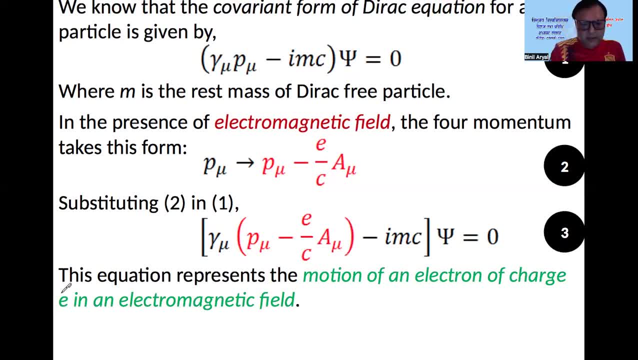 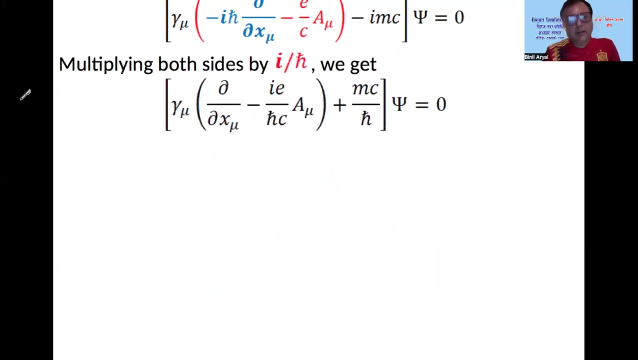 having charge, say the e in magnitude in an electromagnetic field. okay, momentum, momentum, okay, so, so this is the same. uh, abami, uh, let's multiply by this, i by s cot s cot, then you cancel. multiply certain factor, also, multiply moment. non-restrict case. 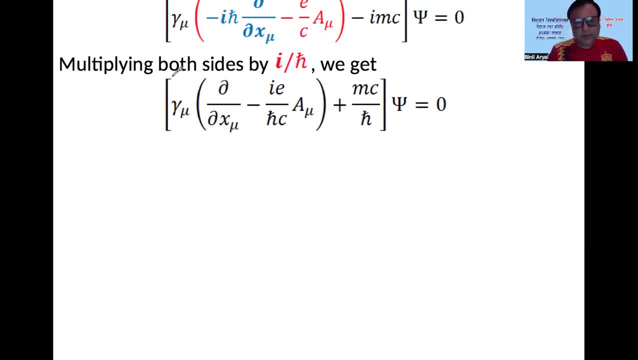 let's, we have multiplied, we have simplified this by taking this operation, multiplication. so we have this form. uh, okay now i mean your mc by s cot, ion mc by s cot, the particular case, particular formula, like the constant, also capital, m size, one layer for simplicity we introduce: 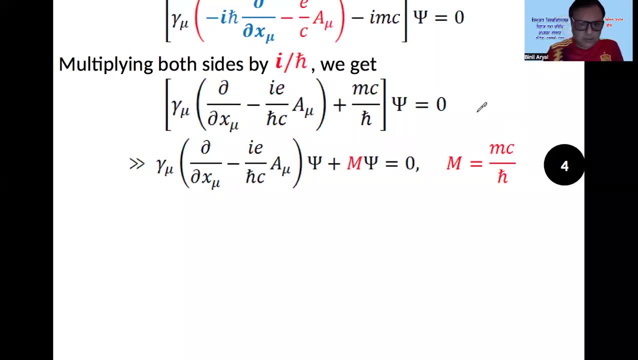 capital m as mc by s cot. okay, so we have this form. what is this? this is nothing. this is direct equation for direct particle which is in electromagnetic field. equation, equation, equation, equation. This is a direct equation of fermion, or of a direct particle which is under the influence of electromagnetic field. 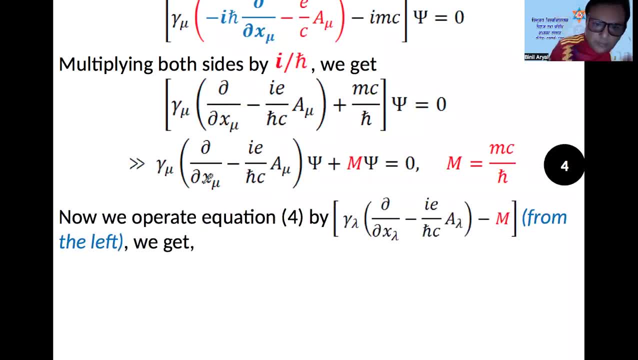 This is a four-vector form. This is a constant form. Constraints are particular to a particular particle. To separate a constant form, we have to move it to the other side and interpret it Directly. we have a form like a plus b. 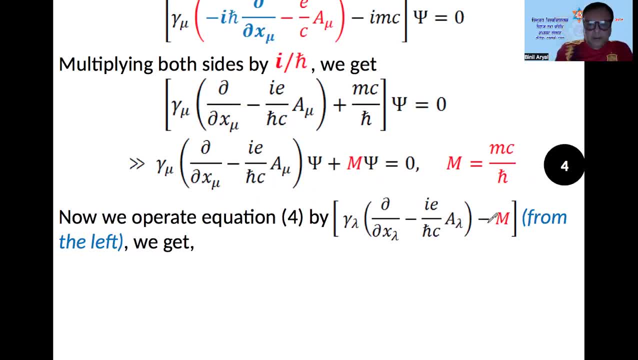 a plus b is operated by a minus b. a minus b into a plus b is a square, minus b square. When it is minus b square we can separate it in a sizable manner. Here it is a square. When it is a square, we can move it to the other side and interpret it. 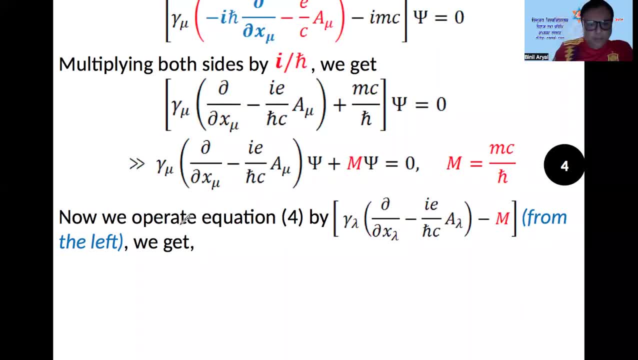 This is a target for every operation. Now we operate our direct-operated equation for this equation by the same, except minus. Obviously that function is operated by someone else. So, from the left, direct-operated equation for by this term. 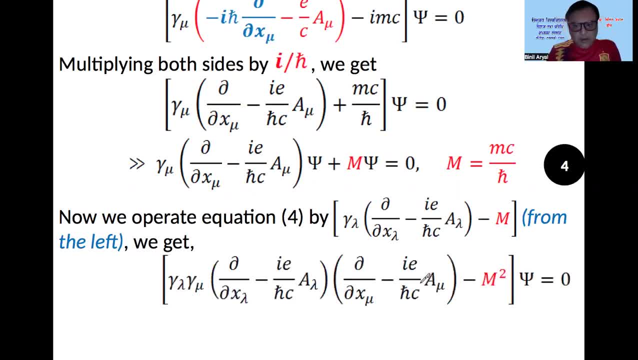 Obviously, the target was To look at this m-square term. if you operate this Now, when we operate this, we have indices. If there is a mu here, it is a lambda indices, So we can discuss it later. 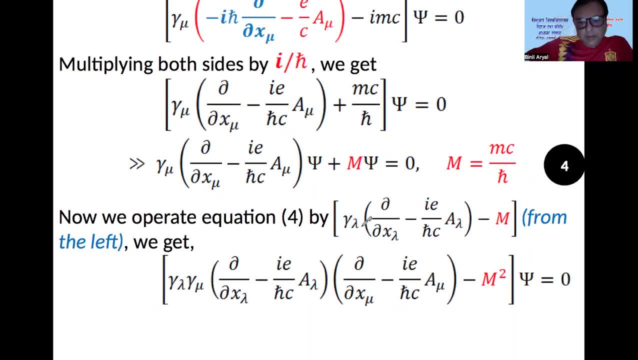 If mu is equal to lambda, or replacing mu with lambda, or if lambda is not equal to mu, what happens? If we can discuss it, we can use different indices, So you have operated this. So here you have a product of this gamma, this 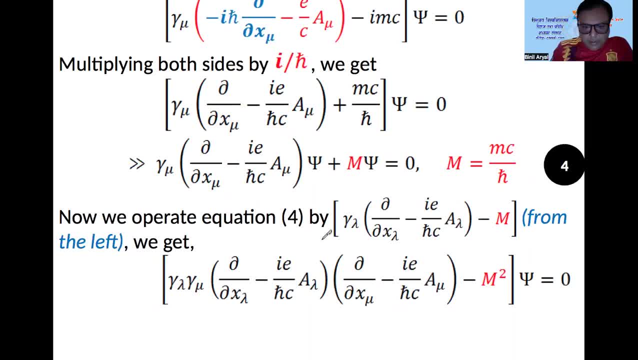 And also this term is for mu. Here you have operated by this lambda term, So this term is here. Okay, This is how we operate. Now we will discuss this term in some other slides. Okay Why? Because we have used these lambda indices. 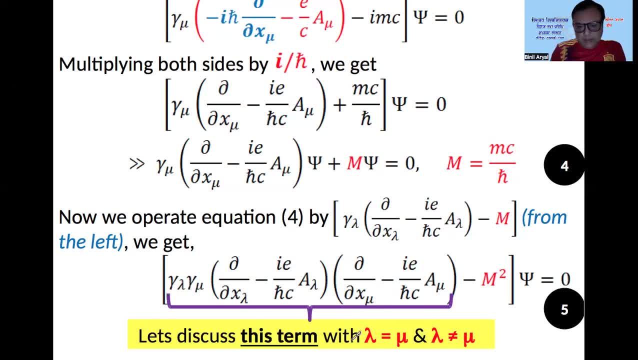 So what happens when lambda is equal to mu? What happens when it is not equal to mu? What happens when it is in the presence of the electromagnetic field? These are the two parts, the spatial and temporal parts. After discussing this, we will separate the spatial and temporal parts. 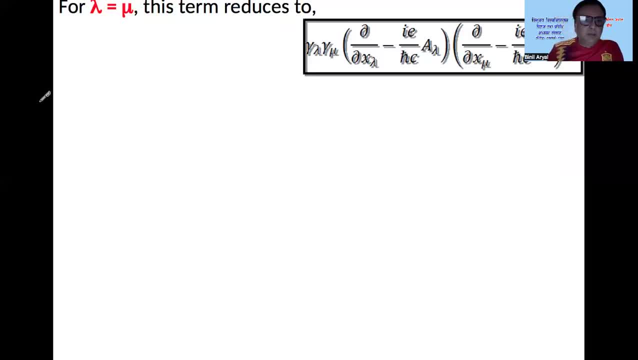 Okay. So let's consider if you replace lambda by mu. Replacing lambda, This term reduces to this term, This term, Your term in the previous slide, This term In the previous slide I left out the square. This term reduces to if lambda equals to mu. 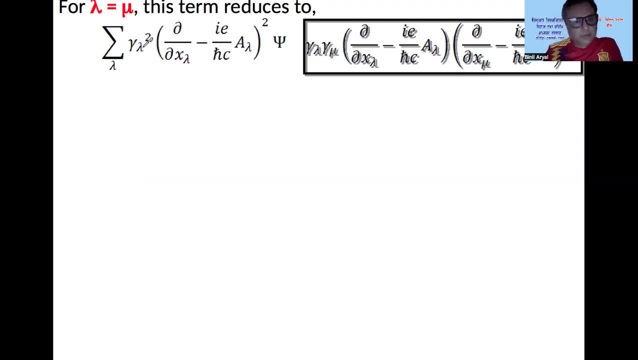 If you write all terms in terms of lambda, then obviously this is a square, And this is also a square If mu is equal to lambda. So this is for a very simple case. You know, this is identity, Or say the one. 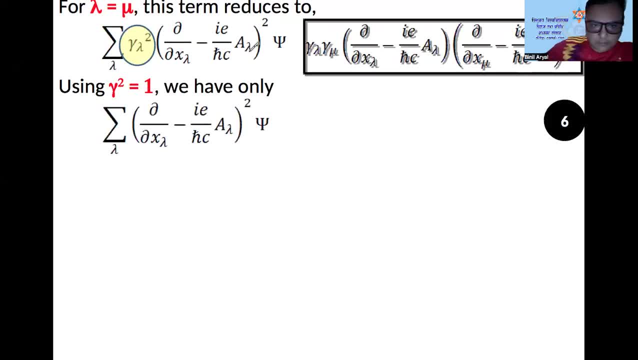 Because you already have function. It preserves the structure of the processes Or the scenario, So you have only this one. If lambda equals to mu, Let's consider lambda is not equal to mu. If lambda is not equal to mu, then you have to take all possibilities to operate each other. 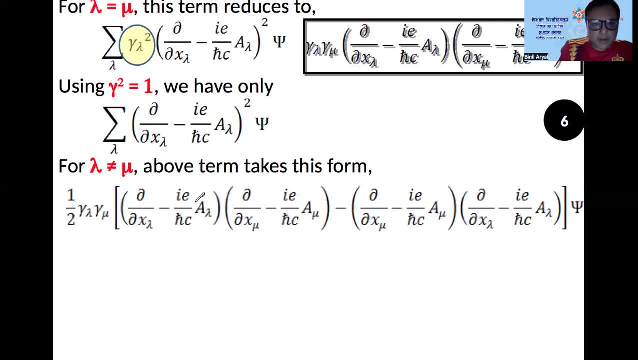 Okay, You can't make lambda equal to mu. You can't make mu equal to lambda. But what you can do is, On one hand, this operator is like this, On the other hand, this operator is like this. And the differences between the two? 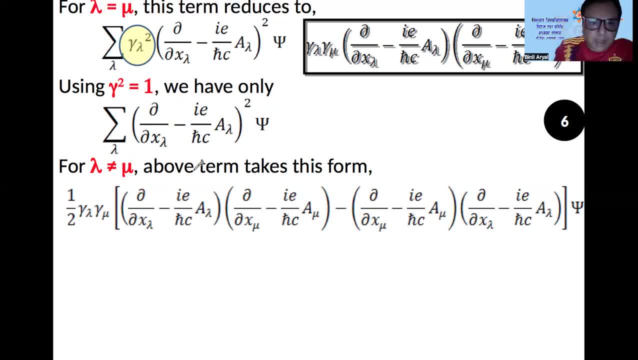 The differences are The difference. There is one here. When lambda equals to mu, it comes. When lambda is not equal to mu, it comes. What additional things will come? These are the things Right. When lambda equals to mu, it will vanish again. 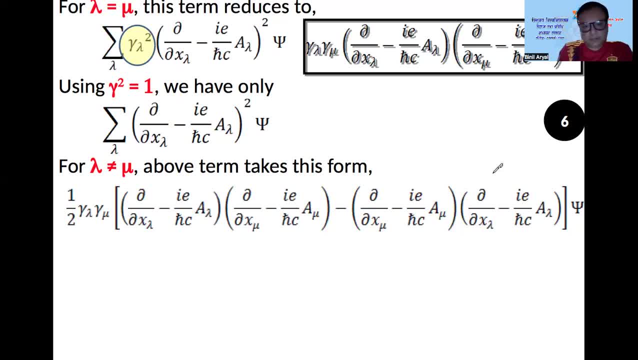 It will be cancelled. These two will be cancelled. When lambda equals to mu, it will be cancelled. Right, And when you are looking at the difference, When you are looking at operating each other, You have to take average it out, Okay. 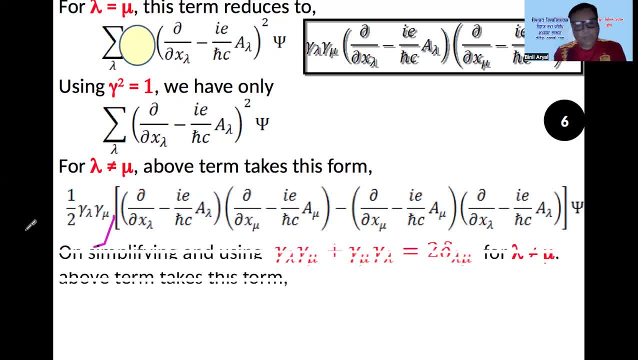 You have to take average it out, Okay, So Now you We need to simplify this equation, You need to multiply this. All are in four vector form, Or say the covariant form. I will, I will, I will. 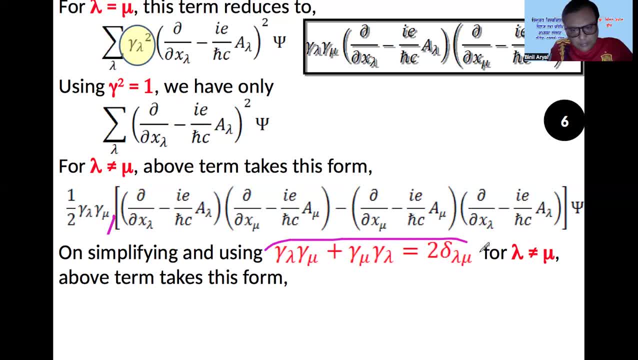 So let's say the equation has all the relations between beta and alpha. So let's write that in four vector form. So let's write that in four vector form. So let's write that in four vector form. Let's write the gamma matrices in four vector form. 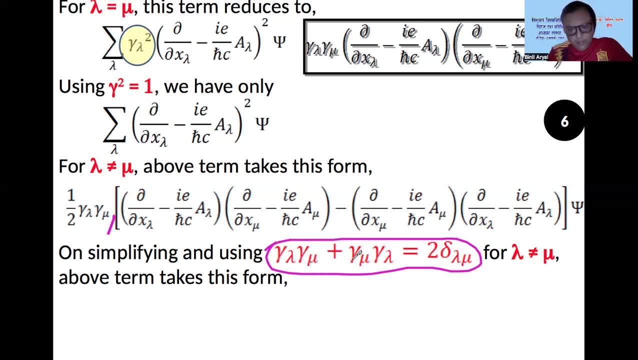 Gamma two, Gamma three, Gamma four, Gamma four, gamma nu. gamma lambda equals to 2 delta lambda nu- This is for lambda- is not equals to mu, So if you also use here so this, then this term reduces to. this term takes only minus half. 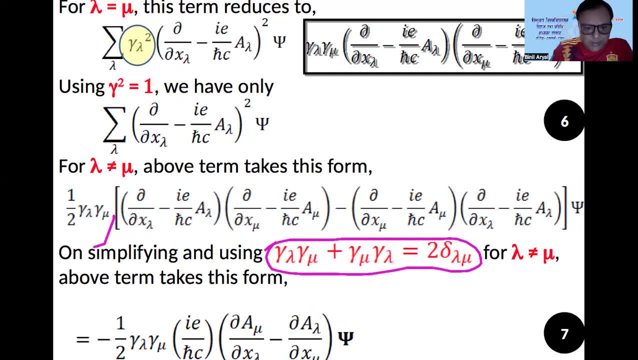 this average out term and you have i e by s cot c from this term and you have only this term d a nu by d x alpha lambda, minus d a lambda by d x nu. So what you have done is: and now what you do is: 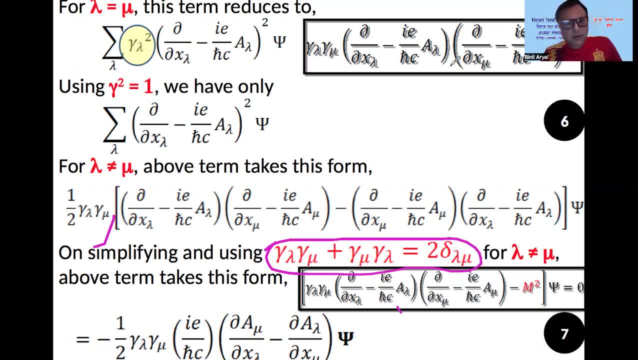 what you have done. You have done these two terms, these two terms. You want to check what will be the effect of this term if lambda is not equals to nu. and you also have. if you replace lambda by nu, you have this term If it is not equals to. 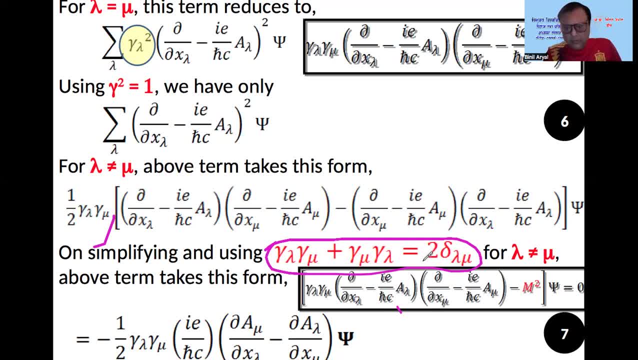 then you have this term, this value. So, in any conditions, whatever the situation for lambda and mu you have, you know the scenarios, you know both scenarios. OK, So now, if you substitute this part in this equation, this is the direct equation for relativistic. 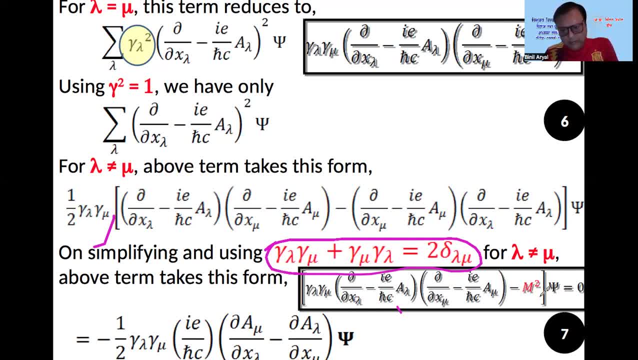 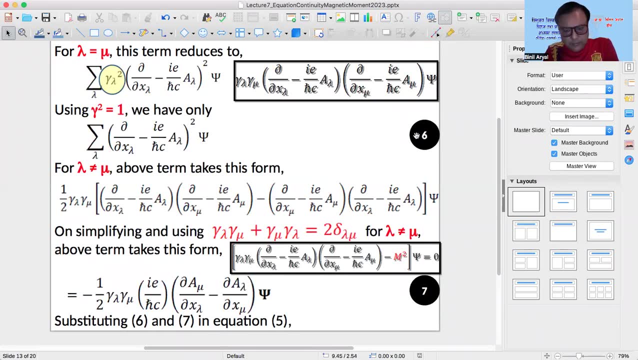 particle in the presence of electromagnetic field. Direct equation, Again equation six: one is substituting. OK, So here I have, I have written substituting equation six. You have an equal Lambda equals to mu. Equation seven: Lambda is not equals to mu. 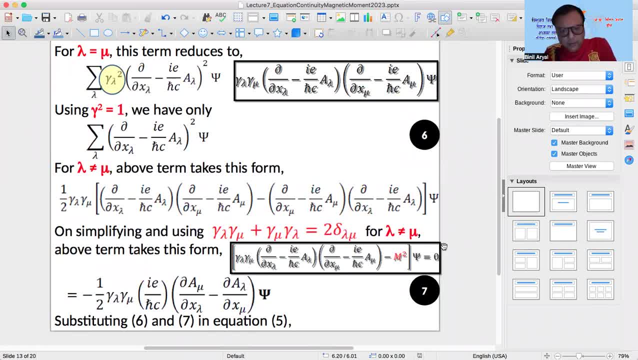 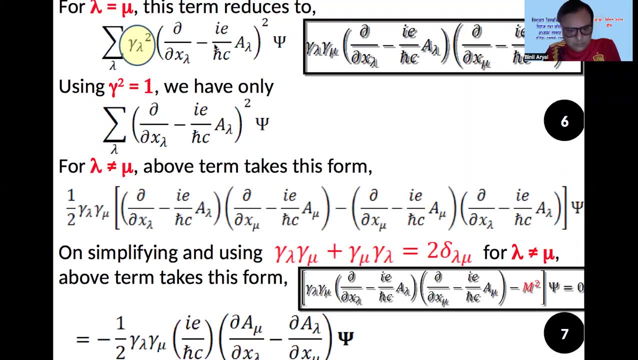 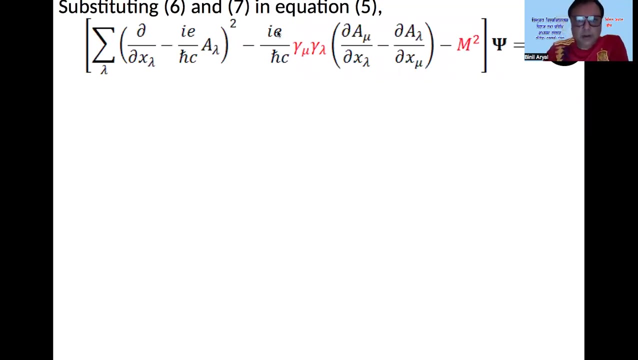 You are substituting these two. Equation five: OK, If you substitute these things here, you get your direct equation. equation takes this form: d by d, x lambda. i. e by s squared. c a lambda square. okay, this is from lambda. is lambda equals to mu. lambda equals to mu, but you are lambda is not equals to mu, but. 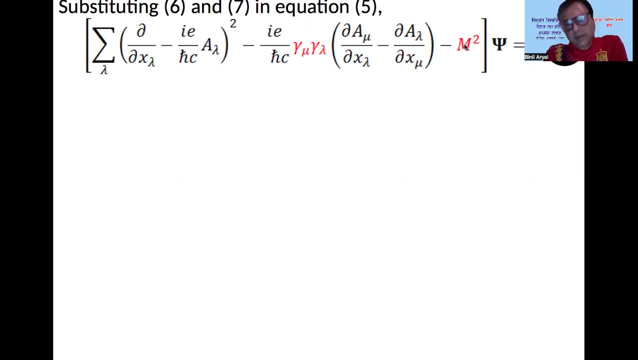 a banky difference and you are okay. i e by s? squared c? u term, then lambda is not equals to mu, but i so do not get confusion, okay. oh, i mean, i have magnetic field is strength. so you look at dynamics del cross. a is vector potential as a magnetic field is strength. del dot h equals to del dot. this. 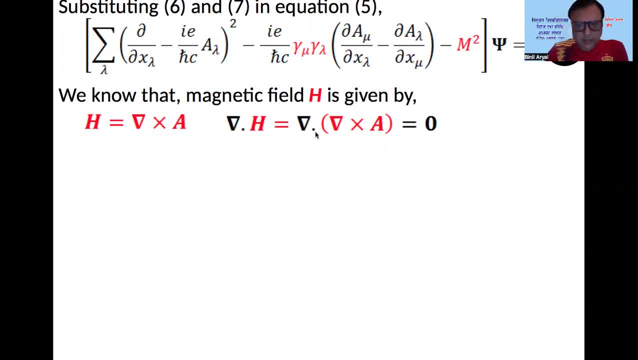 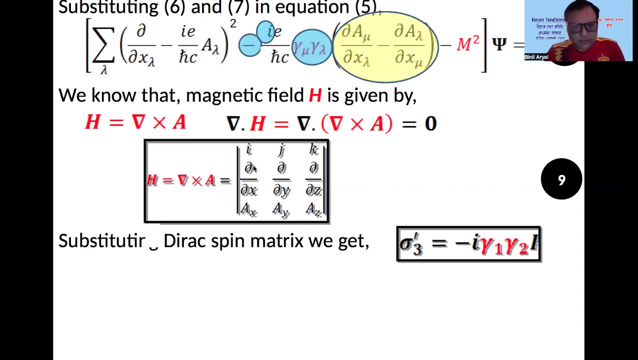 this is the divergence of curl of vector potential is reduced, reduces to zero. you know this and you also know del cross. even if you say i mean a matrix, malik, human, a, h equals del cross, even if i, j, k, and this is for del, d, d, y, d, x, d, y, d, y, d, y, d, z, and this is for last row, is for a, x, a, y and a, z. components of 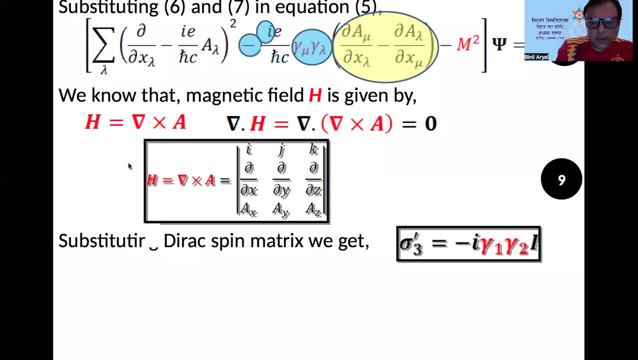 vector potential. okay, oh, I yo- tren qui. ooh, the beginning, richard, a minute mo yo yo here del cross a component. okay, think I gamma, new, gamma, delta you scenario and you mention delta, delta, gamma, new gamma delta. You know, last class I had discussed direct spin matrices. 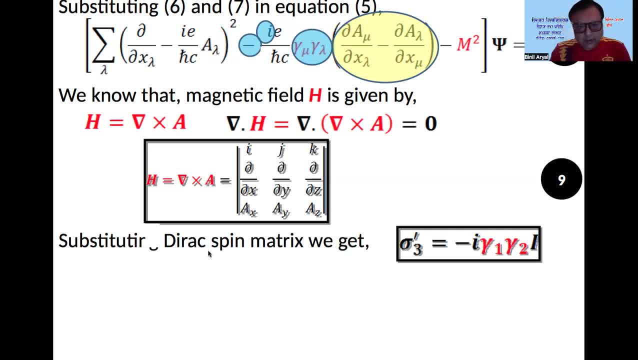 I had introduced direct spin matrices. So direct spin matrices, we know, is sigma prime equals to i, gamma 1, gamma 2, i. This is for third component. Now here, i is there, Minus is also there, Gamma 1,, gamma 2, two gammas are there. 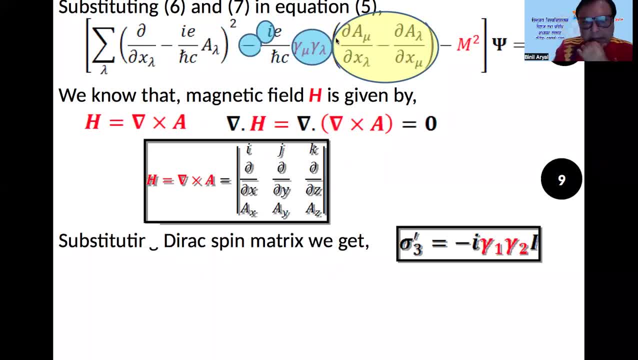 We can make them. This is only error. Identity is given here. Identity problem is not there. So this part here direct spin matrices are replaced, This part here magnetic field strength is introduced. This comes from curl of A, which is H. 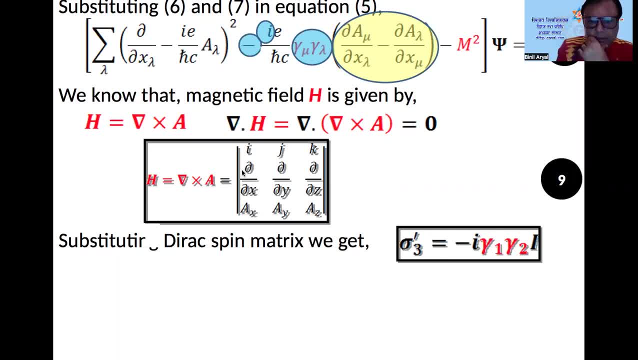 This is A. So here you have A. So these represent one of the components for curl of A. Okay, So your second part: differences are equal, Differences are equal. in a direct spin, matrices are invited. Okay, So if you substitute this in equation 8,, 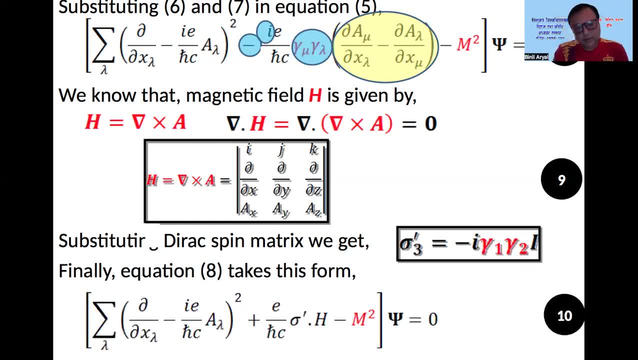 what you get is: first term is the same. Difference is not there, Or lambda equals to mu. is there, It is 13.. Lambda is not equals to mu, So this is left. Minus is there, This is plus. 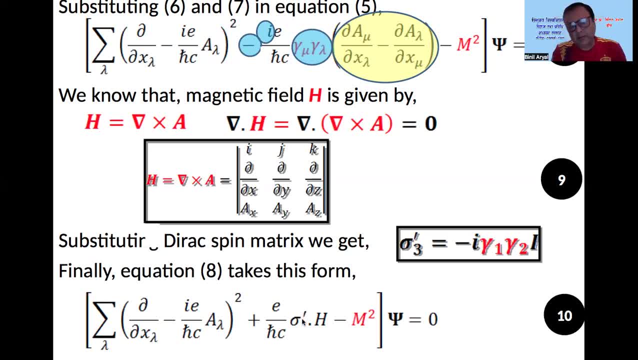 Now here, this term sigma prime is the same as sigma prime. This is direct spin matrices. Dot H: This is H. H is there? So you have very beautiful term. This term contains direct spin matrices. This is the magnetic moment. 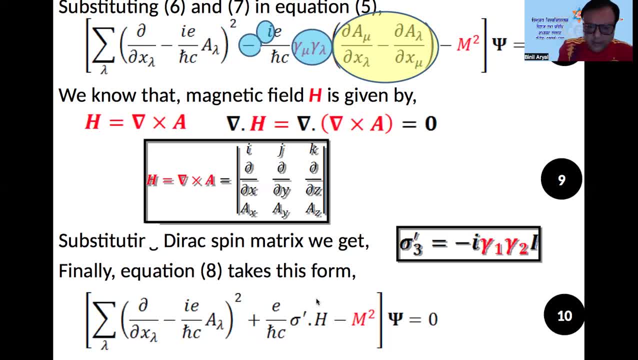 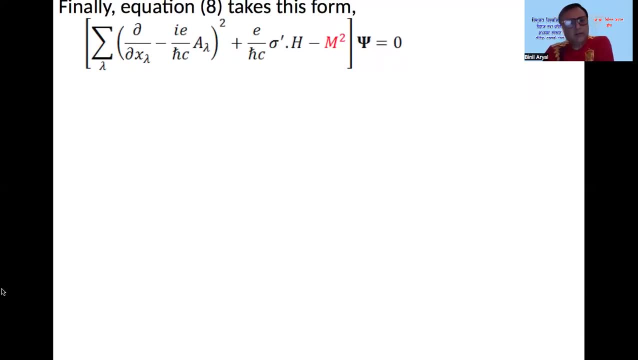 turning effect. Turning effect is accountability, linear term. You can write it successfully. You can write it successfully. Now, derivation is sigma prime, The expression. you can write it easily. Okay, Its derivation is a bit tactical. This is the same equation. 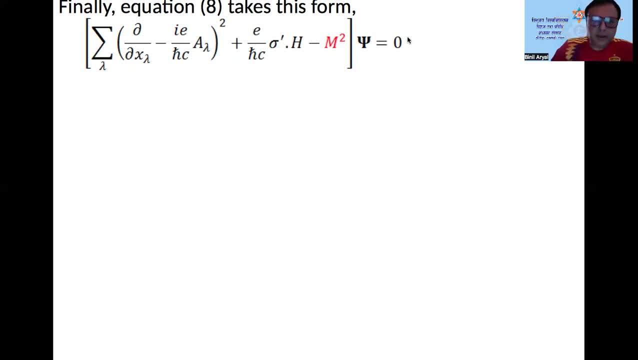 This is direct equation In the presence of the local magnetic field. we have written this equation in terms of magnetic field is strength and vector potential. Okay, So now this in particular: there is a vector form here. Let's separate it. 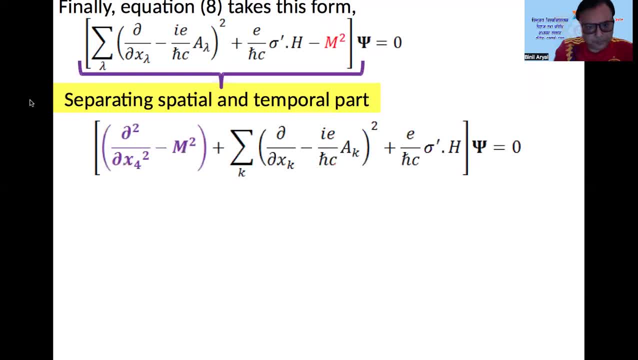 Separate the spatial part and the temporal part. Okay, I will try to explain it a little bit. OK, let's separate the spatial and temporal parts. Now look here: in lambda, the x, y, z is the spatial part and t is the temporal part. 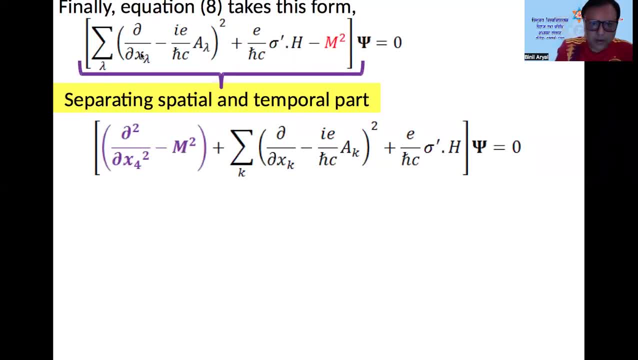 So t is x4.. So the temporal part of d by dx squared is x4.. So the first part is the temporal part of t squared. So it fits with this. OK. Now there are several other terms that multiply in several ways. 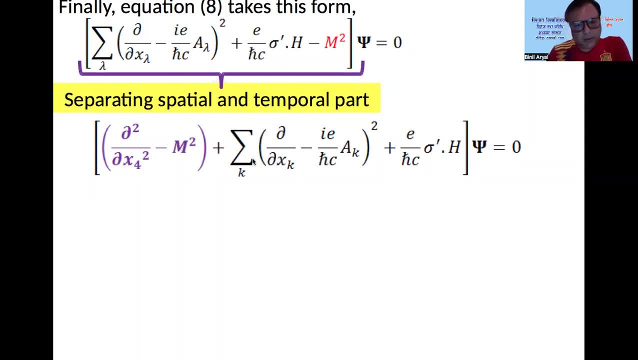 The ones that are systematically multiplied. the three components: k is the spatial part. We have written the rest as sum over d by dx, k. here k runs from 1 to 3, 4 is here. OK, So Ie by h squared, c is here. 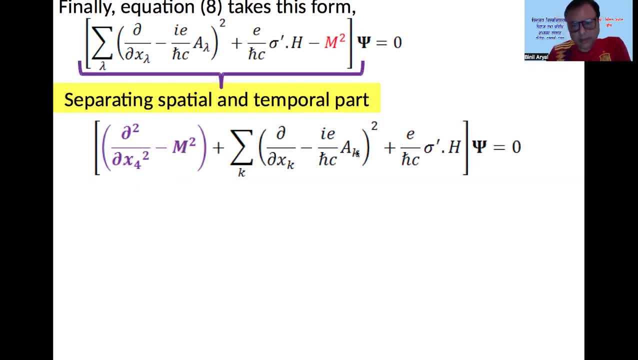 So here also, you have only the three components k, The spatial part is here and the temporal part is here. OK, So this is the term that you have obtained. That's why I made this the spatial and temporal part. OK. 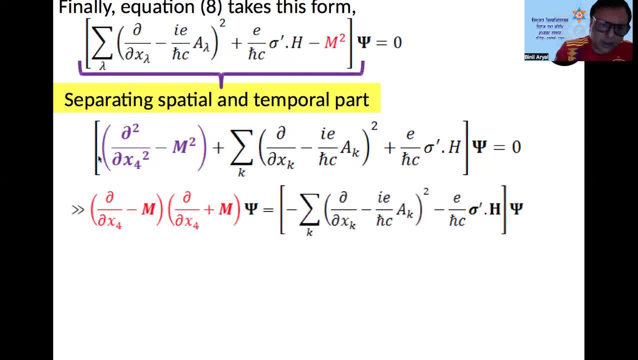 Now what I am going to do is I am going to write it in the form of a plus b into a minus b. Here, Right, And here. it is the same. It is just separated. I am going to put it aside. 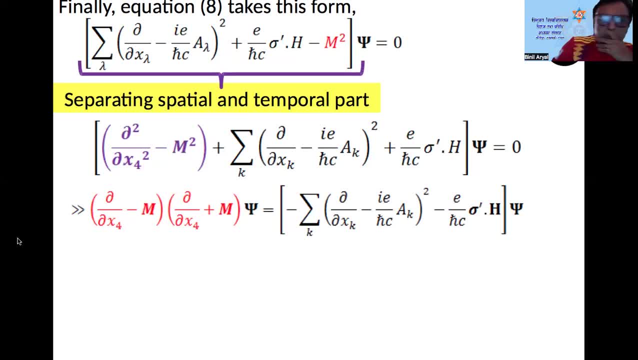 OK, Now in the derivation of the following: how to find the value of direct and contemporary moments, How to address the direct spin matrices, How to find the experimental value. So I think, exactly in the figures. there were many attempts But ultimately, 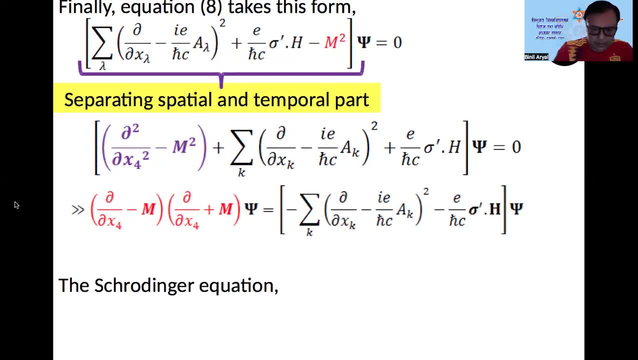 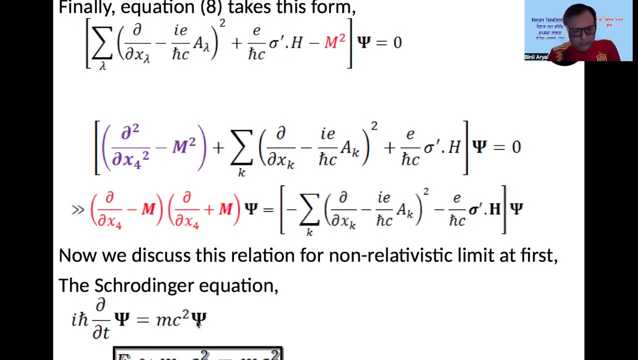 based on the quantum mechanical postulates. what could we do? OK, Now we will discuss this relation for non-regulatory limit. first, Let's go to non-regulatory limit. We know the Sogno equation: Ie by dt equals to: 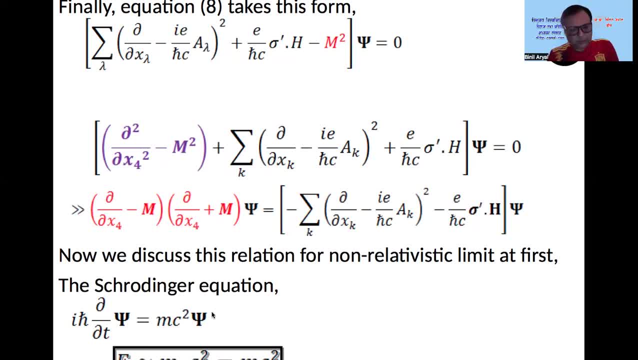 let's say e psi. Let's say e is mc squared. So this is Sondre's equation for particle having energy mc squared. Again, I multiply above c and below c And I take the above, i below. here To adjust this, I take i square minus i. 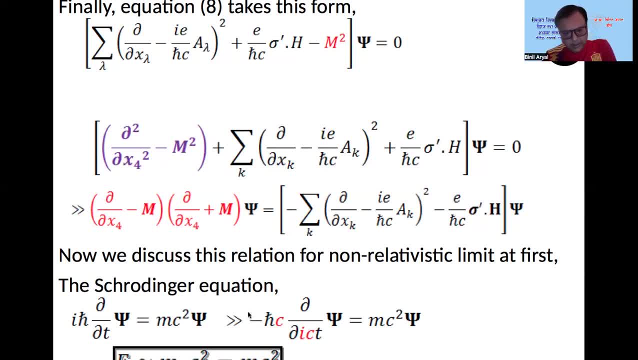 So this minus indicates i square Here one. i gets cancelled and you have this one. So here you have ICT. This is actually x4.. This is d by dx4. psi Equals to cc, or cc is cancelled, so it is divided by s squared. 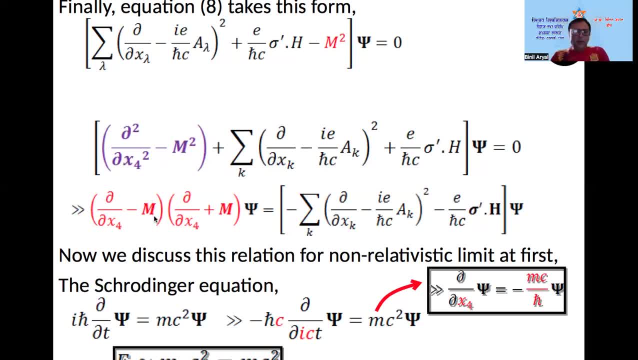 This is exactly what we came up with for m. We considered m as mc by s squared. We considered mc by s squared, So you get more or less similar term. So mc by s squared is capital M actually in your case. 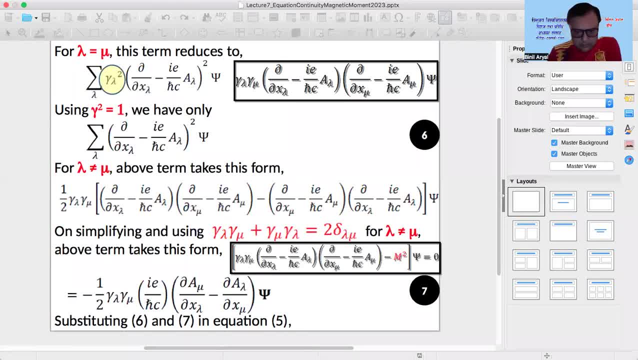 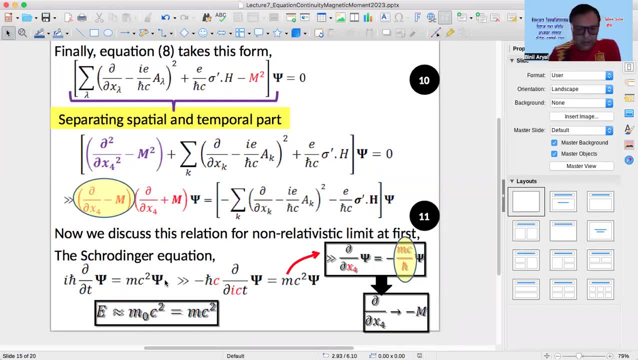 So here this Sondre's equation for the particles that have energy equals to mc. squared gives this term: d by dx4 psi equals to minus capital M psi. Now what is d by dx4?? d by dx4 is equal to minus M. 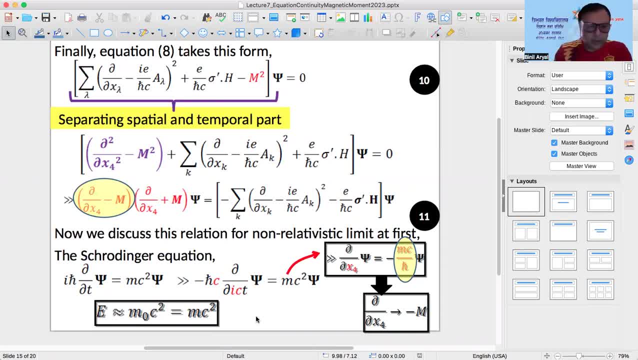 d by dx4 is equal to minus M. Now if we put minus M in the place of d by dx4, if we put minus M here, then minus M gets cancelled. This becomes zero. It becomes zero here, So the contribution of the temporal part is lost. 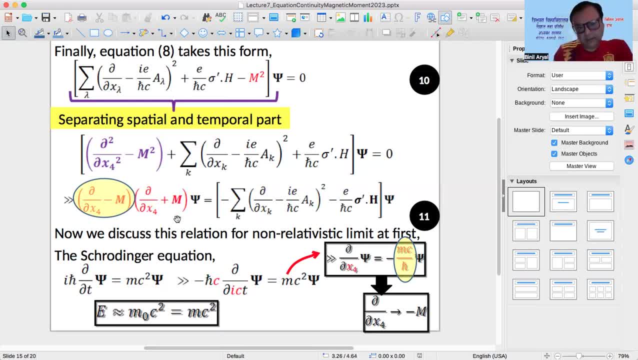 The contribution of the temporal part is lost. The contribution of the temporal part is lost, And directly what we do is: d by dx4 is here and here and here, but the d by dx4 that is here is the only one that is minus M. 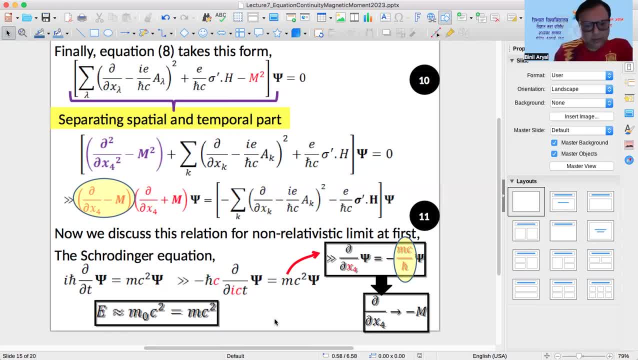 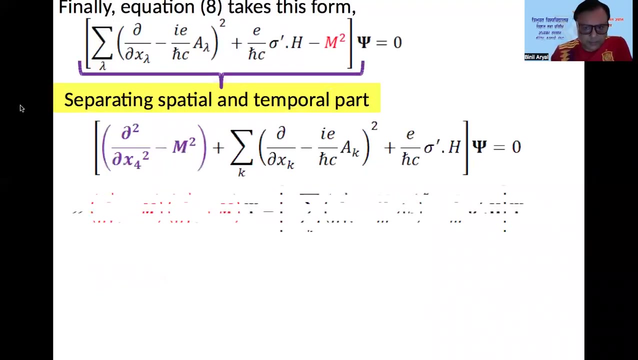 Considering this relation. So this is not for the non-heuristic particle. This is for the particles that have energy equals to mc squared. This is for the particles that have energy equals to mc squared. OK, So here we don't have any of these steps. 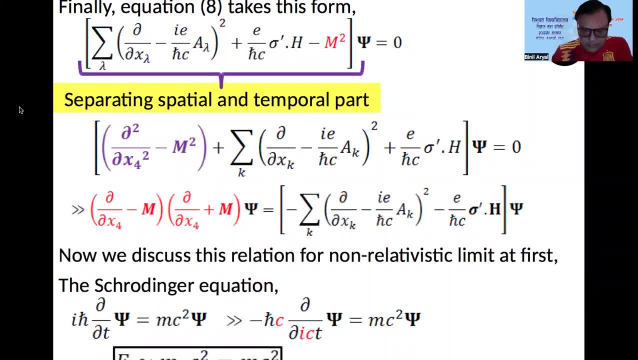 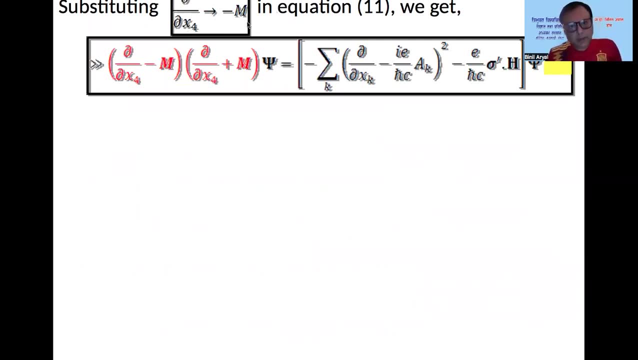 just these ones, So we still have more language to explain. OK, Now I will go to the other slide again, And directly is actually minus m, then d by d. x will be kept here only. If kept here, then already it will be cancelled. 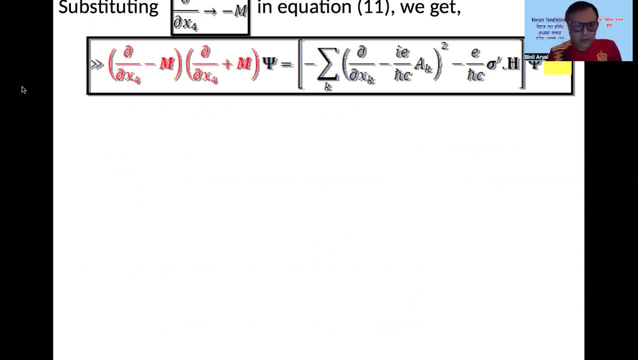 It will be a special part only, Right. So he has inserted minus m here. So in this way you get minus 2m from this term and you have remaining this term, d by d x plus m. So simplifying this. 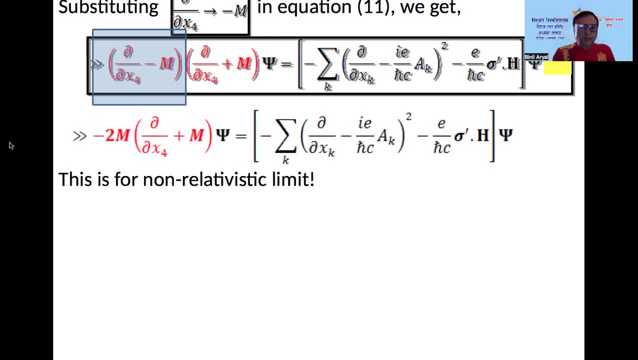 so this is actually he has written. this can go up to non-linearistic Equals to mc square's value. even if you put it together, it will still exist Because in this term which was imposed, c's value. 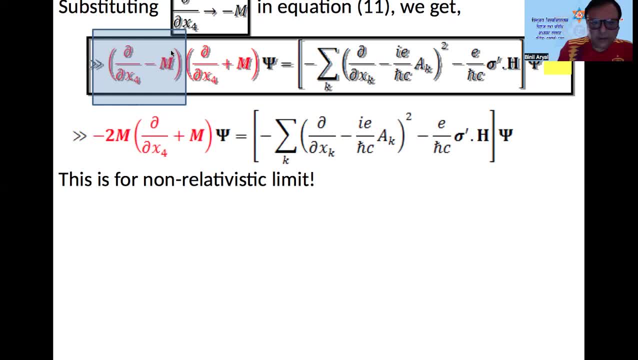 is exactly. if it is less than the velocity of light 0.9c. 0.8c, it is also applicable. So this moves to. this is called. this equation moves to the or concides can concide. 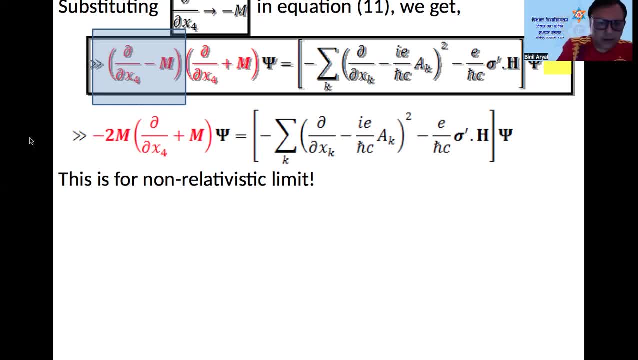 or should concide to the non-linearistic limit. I have written it. Okay, it is not yet excellently verified, not verified. So this is for non-linearistic limit. So, just simplifying this, let's just multiply it. 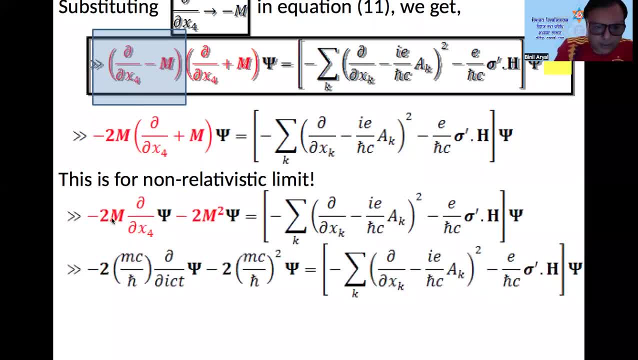 Okay, Then m we know, mc by h square, this right, the values of m here and values of m. mc by h square, mc by h square: here we have kept real values. We have kept real values. 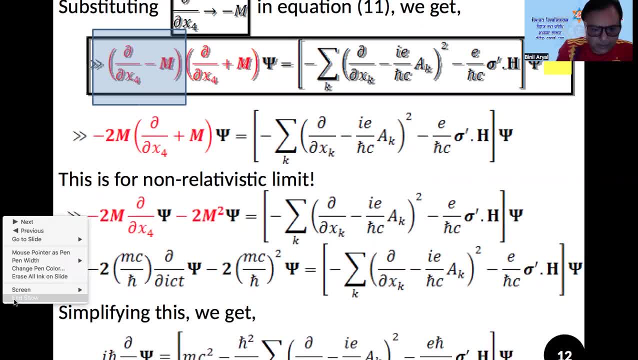 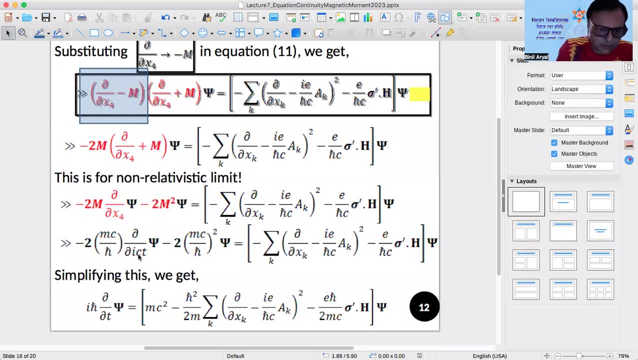 and we have simplified them. By simplifying we get this kind of correlation. You know that is d by dt term. I see, and so you get. if you simplify this, you get. I has got d by dt. 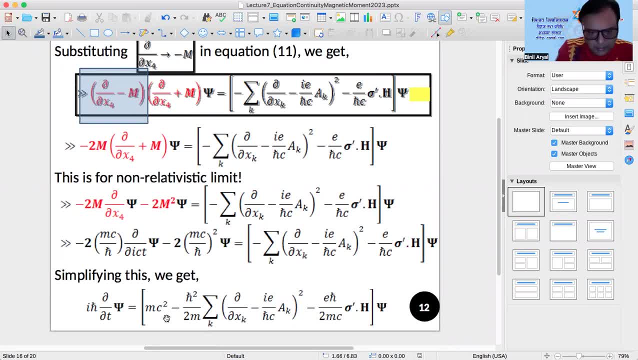 psi. I has got d psi by dt, equals to h psi. I has got d psi by dt equals to h psi. So this h, this Hamiltonian, is for the direct particle under the influence of electromagnetic field. Okay, 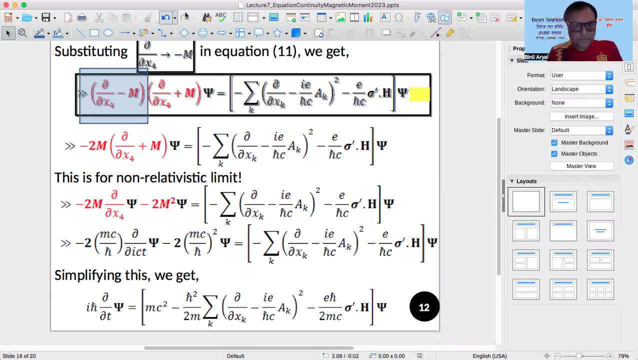 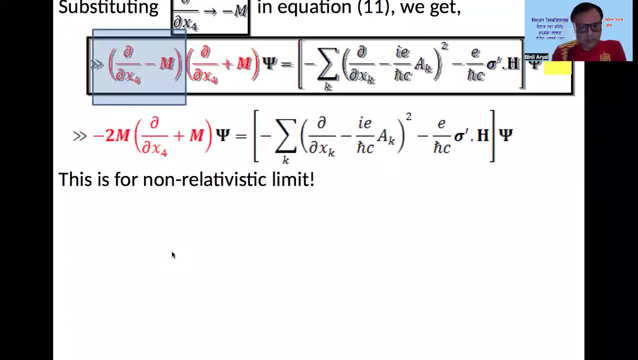 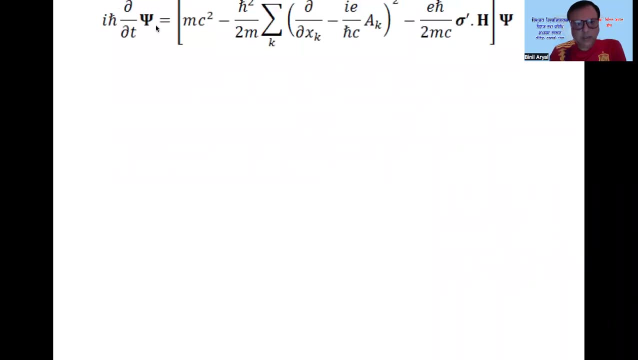 So here this is for the direct particle under the influence of electromagnetic field. So this is, I has got d psi by dt equals to h psi. So you now you know what is h for direct particle in the electromagnetic field. 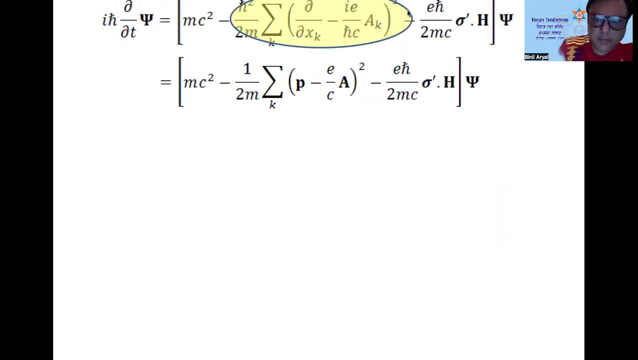 Now, if you reverse, if you go reverse, I mean if you go back, I mean if you insert the effective momentum, like what happens is 1 by 2m or p square by 2m, no, 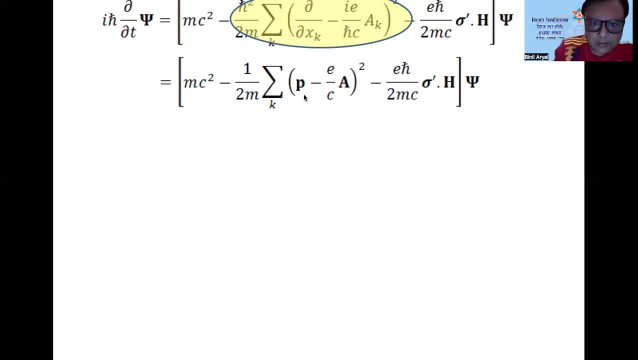 p square. this is p effective square. So this is p effective square. So, if you go back to the, the terminology that we have used in used for non-reactivistic quantum mechanics, So this term is simply this one. 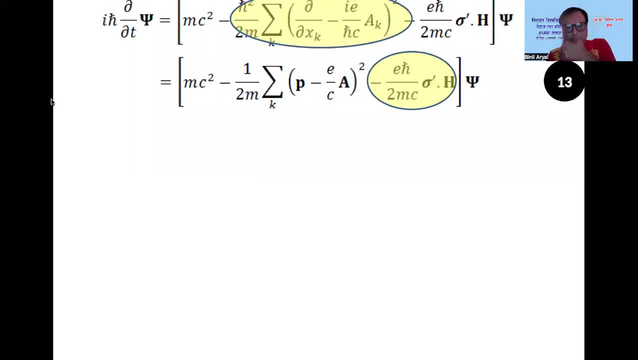 and the remaining terms are same. And here you see, this is the relativistic energy, This is the kinetic energy under the influence of the electromagnetic field. And what is this? This term is responsible for turning effect, Just like we had done in the previous generation. 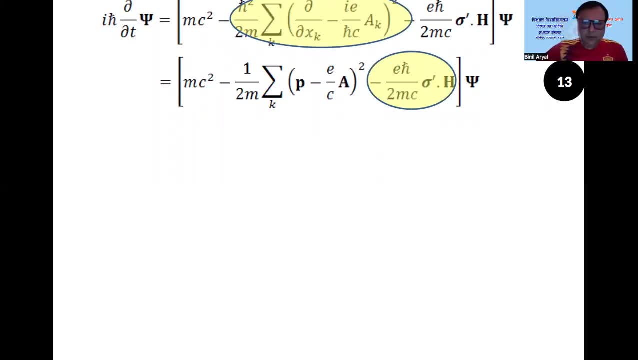 the term of self energy had come. this is the turning effect. the term of the magnetic moment. this is the term that had come. this is the term of kinetic energy and potential energy. we have removed this. this is a particular term. 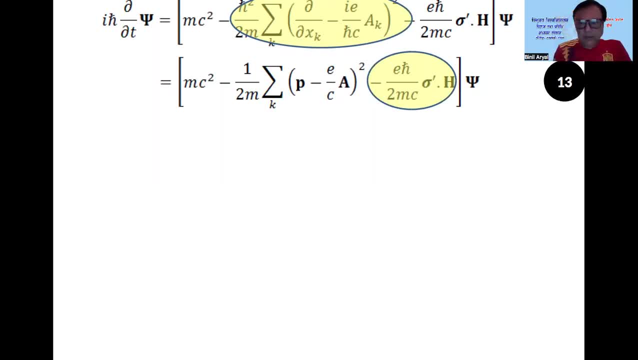 a term that can only be turned. What we have seen in this is the term that can be turned. is this in Hamiltonian: Okay, So you know that the potential of a magnet, of magnetic moment mu in a magnetic field is minus mu h. 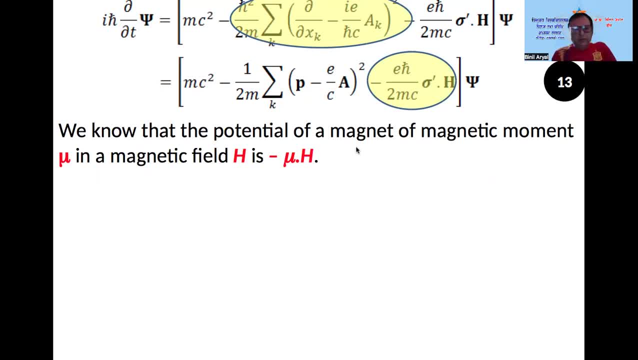 So this is in all cases in classical mechanics, also in relativistic quantum mechanics, but you put in relativistic, in non-relativistic quantum mechanics you put magnetic moment for electron due to its precision. Okay. So this equation. 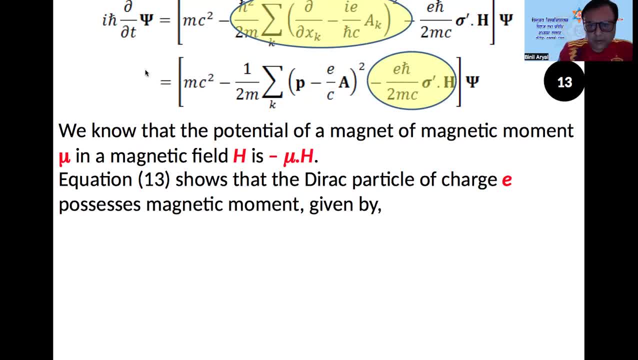 13 equation in which you have Hamiltonian and in the Hamiltonian you have a term that is responsible for: to provide magnetic momentum for the relativistic particle. This shows that the direct particle of charge E processes possesses magnetic moment. 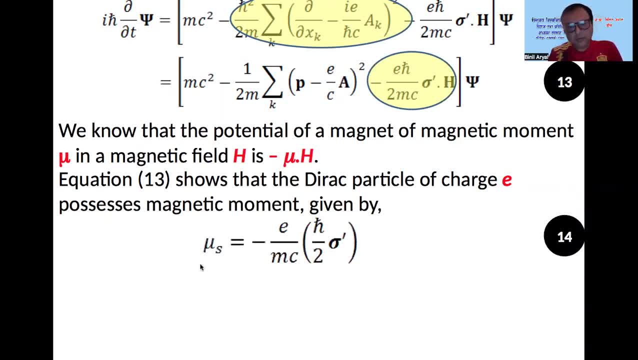 which is given by this term. So this is the magnetic moment for relativistic particle or for direct particle under the influence of a local magnetic field. in the presence of a local magnetic field which is as caught by mc 2mc. 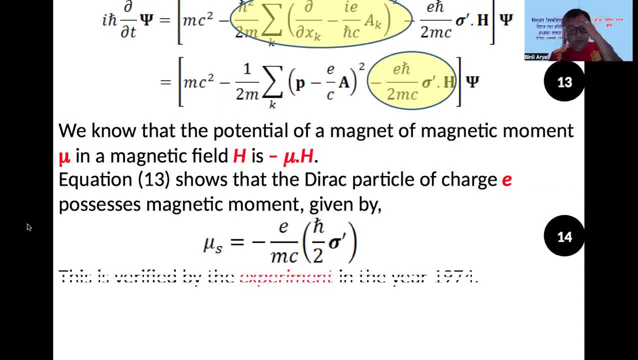 sigma prime. Sigma prime is direct spin matrix, So this is experimentally verified. It's not only a value, it's a value that came before. It's a value that came after the experiment in 1974.. Okay, This is experimentally verified. 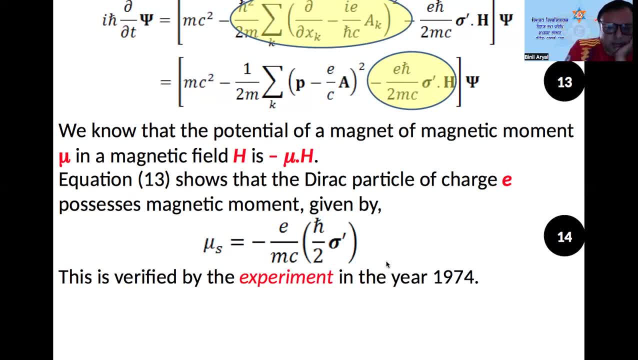 but this was 1950s and it came before that theory. There was many other. in this expression you have to replace m by this relativistic part. The real experiment of the rest mass does not have a rest mass, So you have to replace this. 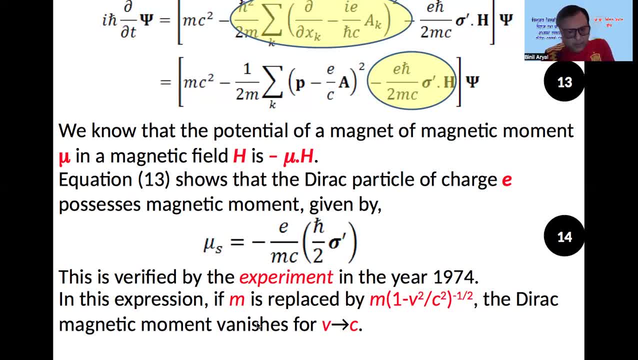 You have to do calculation And the direct magnetic moment vanishes. for if it goes in the same velocity, the direct magnetic moment vanishes. The velocity goes in the same velocity. the mass is infinite. If the mass is infinite, the magnetic moment is zero. 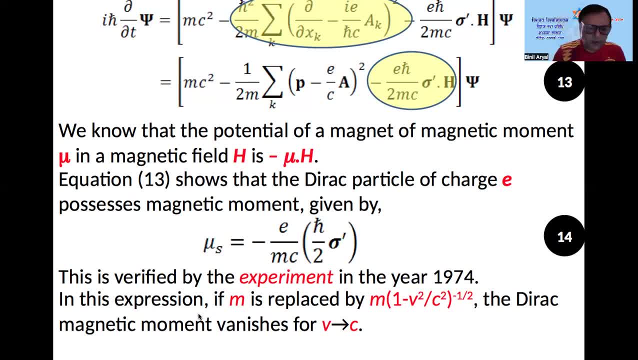 Okay, So you should remember this: Direct magnetic moment, or magnetic moment for direct particle, vanishes if the speed of the direct particle is exactly or coincides with the speed of light. However, that is not possible. It will be less. 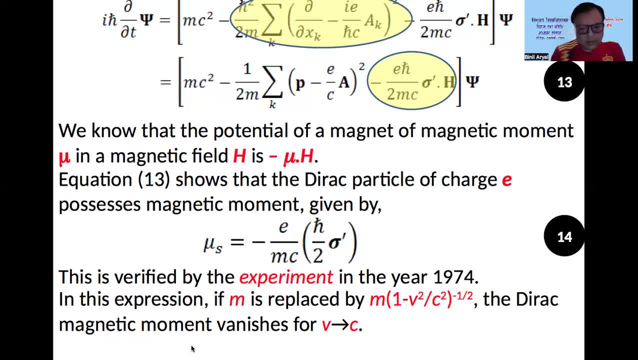 If it is less, its magnetic moment will exist. It will exist. Direct magnetic moment appears only in non-realistic limit. Obviously. I mean non-realistic limit means if it is less than c, then your limit is gone. Okay. 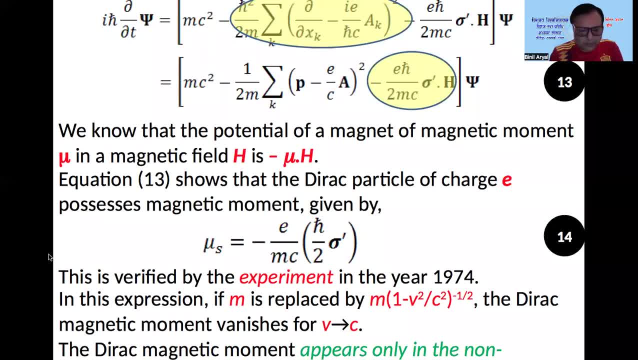 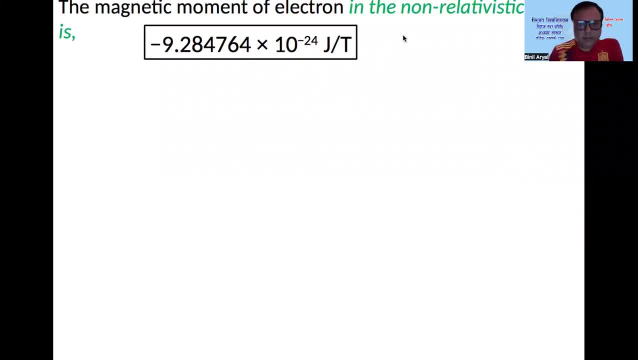 And if it is less than c then the magnetic moment will exist And also it depends on charge. Now we have seen in the previous class we saw the value of the normal, non-realistic quantum mechanics In the first semester. 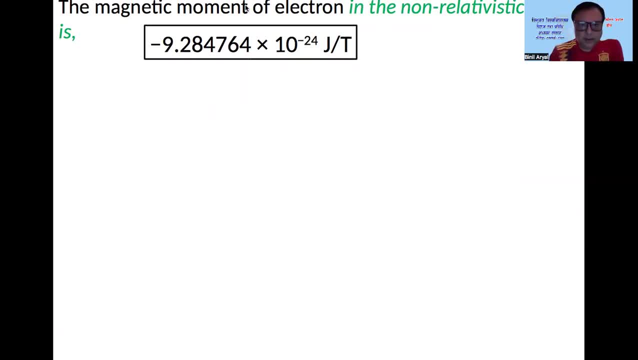 we saw that the value of the magnetic moment in precision is electron. The mirror of the nucleus is the electron. The charge particle is the electron. The charge particle is motion. The magnetic field is created. The electron produces its own magnetic field. 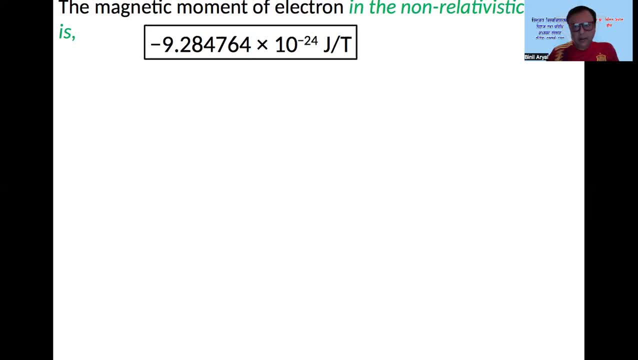 If the magnetic field is replaced, there will be a magnetic moment in this order That is like a joule, And the relative magnetic moment. then this magnetic moment is observed by a small magnetic moment. It is called anomalous magnetic moment. What is anomalous? 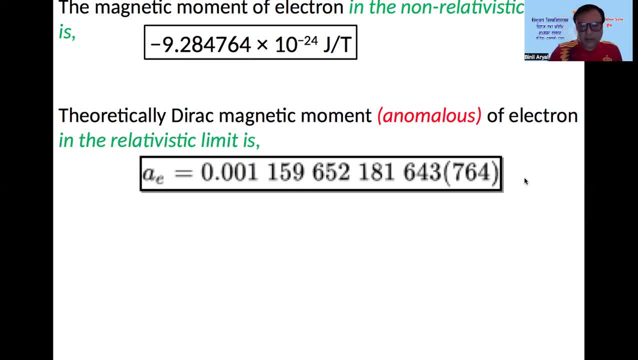 It is the effective magnetic moment produced by the relative stick. Anomalous, non-relativistic, pure non-ladivistic will have a magnetic moment, as it is said today. We have to understand this by saying this: This is the unit of the ratio. 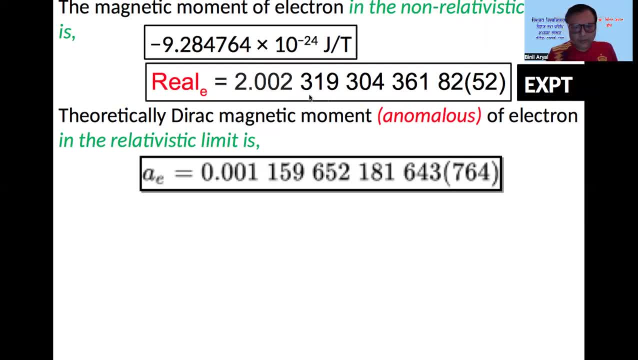 If we write it in this unit, it is 2.003319 and so on. So this is the magnetic moment of non-ladivistic electron in this unit. But if the electron is relativistic, becomes relativistic approaches to relativistic. 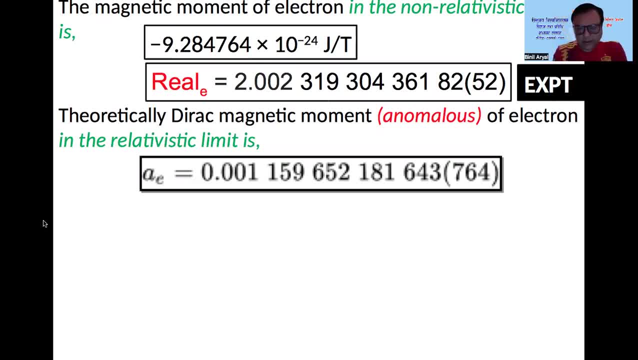 then another magnetic moment appears That is called anomalous magnetic moment. If you compare with these two, this is very, very small. You see this is 2.002.. Here it is 0.001.. That means 0.001 by 764 digits or so of absorbance. 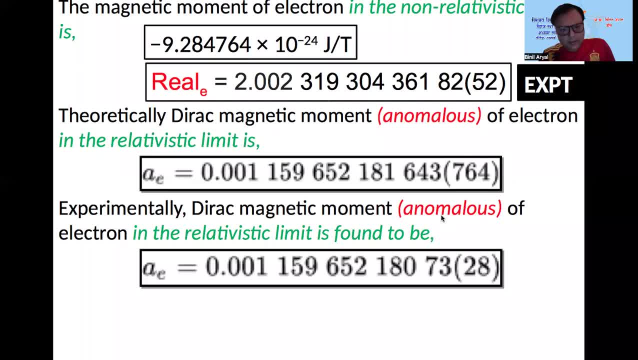 Experimentally direct magnetic moment electron of electron in the relativistic limit is found to be: This is the experimental value obtained from the lab. This is the theoretical value calculated using the equation that we have discussed in the previous slide. Okay, So there is a very good agreement between the experimental result and theoretical result. 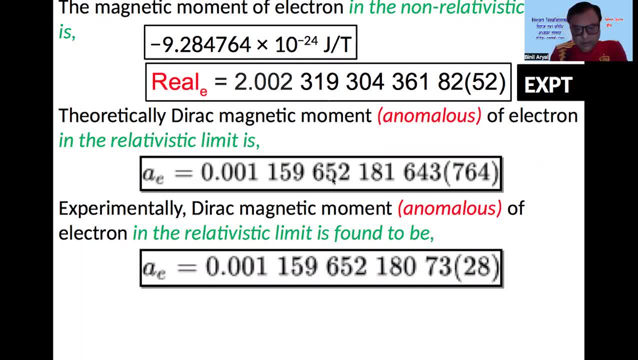 You see 0.001, 159,, 159, 652, 652.. The difference begins from 0.001.. The difference begins from here, after 10 digits: 181 is here and 180 is here. The difference begins after 18.. 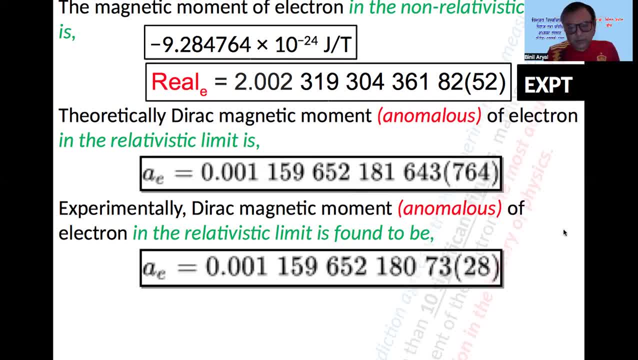 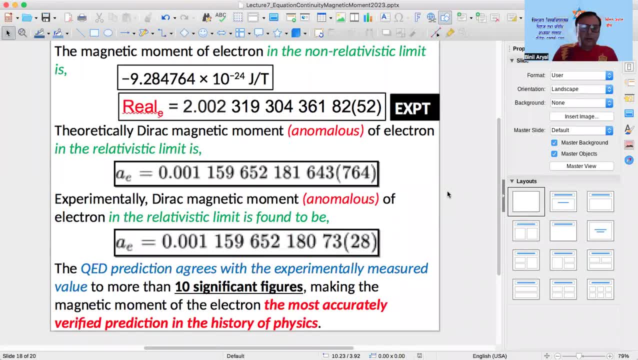 Okay, So this is a very interesting agreement. This is a very good agreement. By making this agreement better, the prediction of quantum electrodynamics, QED, is satisfied. The QED prediction agrees with experimentally measured value to more than 10 significant figures. 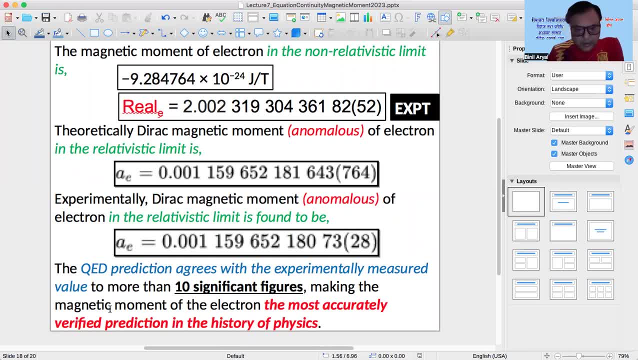 More than 10 significant figures Making the magnetic moment of electron the most accurately verified prediction in the history of physics. Most accurately verified prediction Up to this high level. there is no agreement between theoretical value and experimental value. There is no difference between physics. 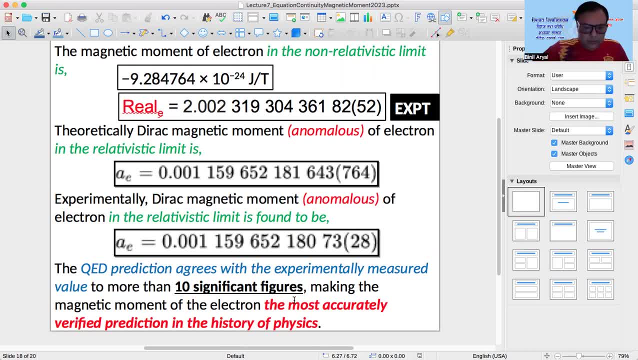 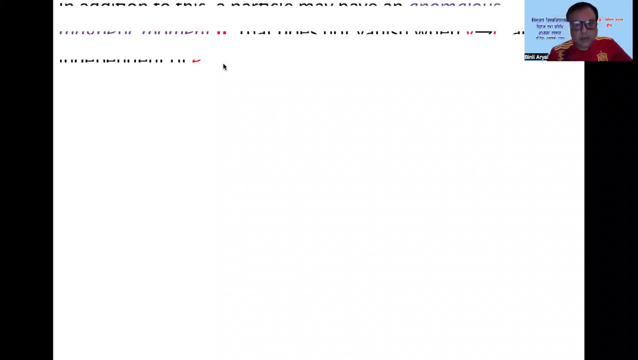 Up to this high level, Right? So that's why it is said that it is the. this is the most accurately verified prediction in the history of physics. Okay, So, Okay. Now for the anomalous magnetic moment. it is written as Ua. 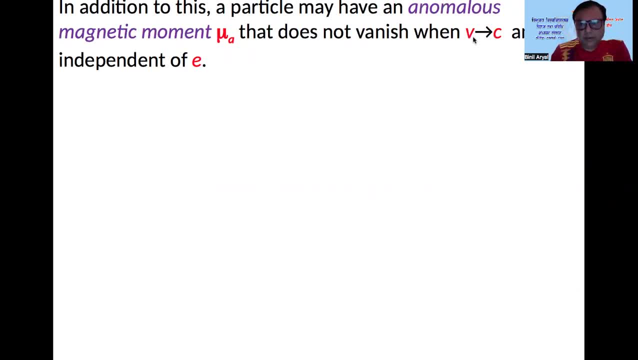 Right, That is, that does not vanish when V tends to zero. Earlier we said that when V tends to C, the magnetic moment vanishes. But even when V tends to C, the magnetic moment does not vanish, is the prediction. 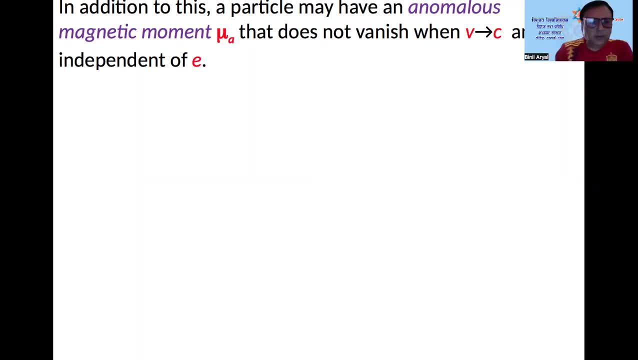 There is a theoretical extension. It is not in our course, but I will write this in the slide. Pauli included the term- I will include this term in equation 8, to describe a particle that processes, processes, processes, processes. 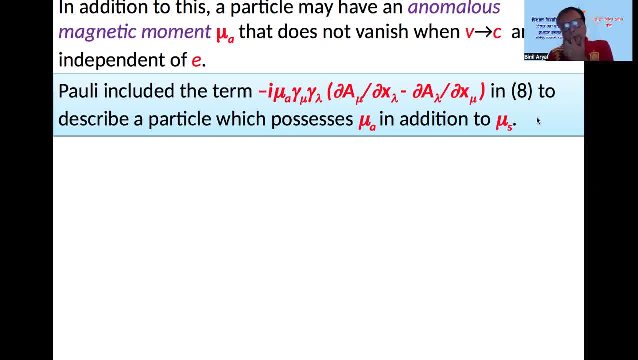 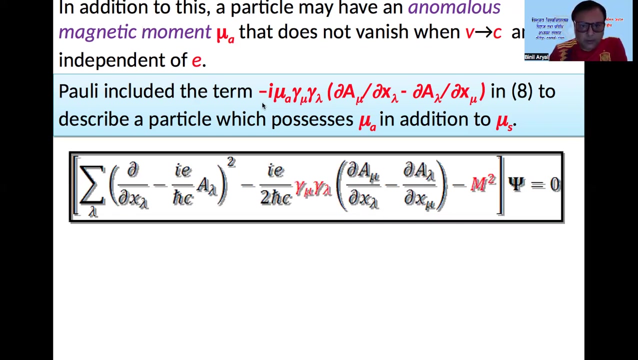 processes, Ua In addition to Mu-Yes, We have been discussing apo-C's, the magnetic moment due to the relativistic spin, to the spin of the relativistic particle That is. I must say, In this way we can include the term minus i, mu A in 8 to describe a particle which possesses an anomalous magnetic moment. 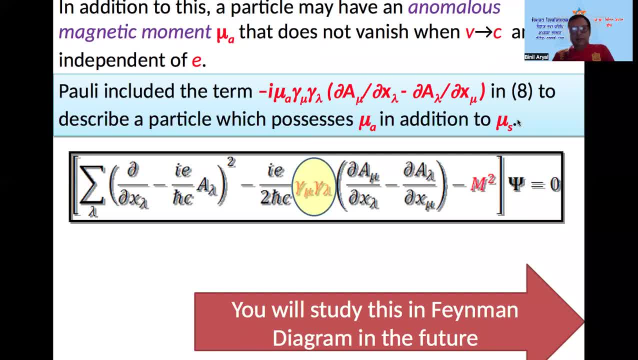 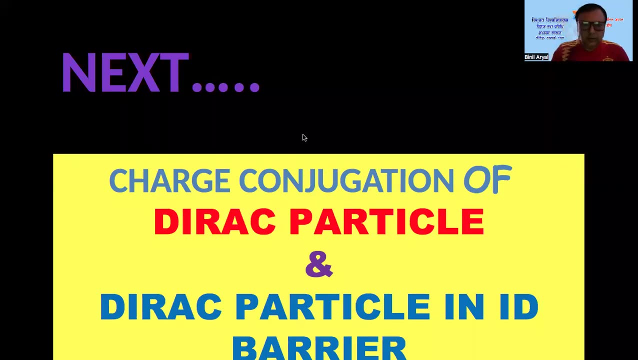 This extension is slightly applied in Lagrangian density. It is read in the Fenneman diagram formulation. So you will do it later. So just remember this: Do not write in the examination this part. OK, so in the next class I will discuss charge: conjugation of direct particle. 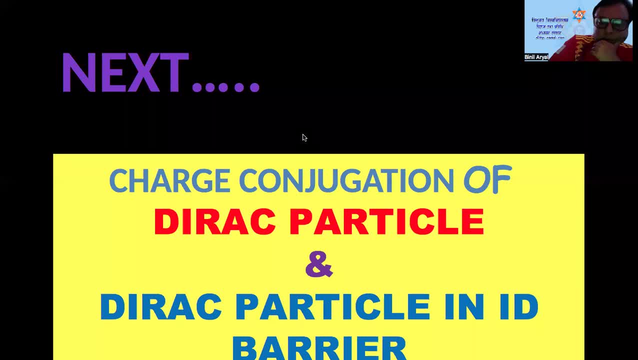 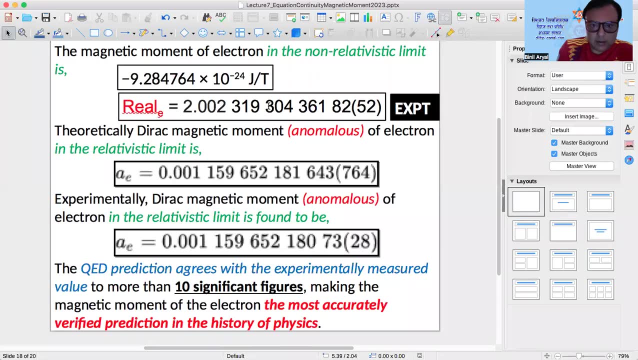 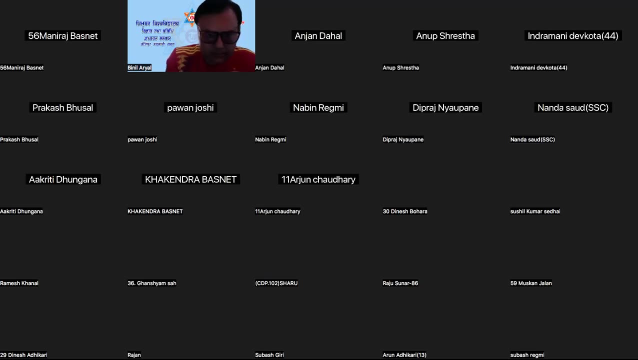 as well as direct particle. conjugation of direct particle. Direct particle in 1-D box, one-dimensional barrier or box. OK, OK, I have kept a slide. You can ask me questions in the next class. You can mail me questions.